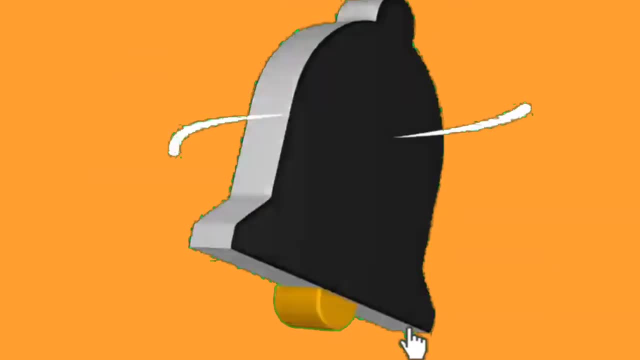 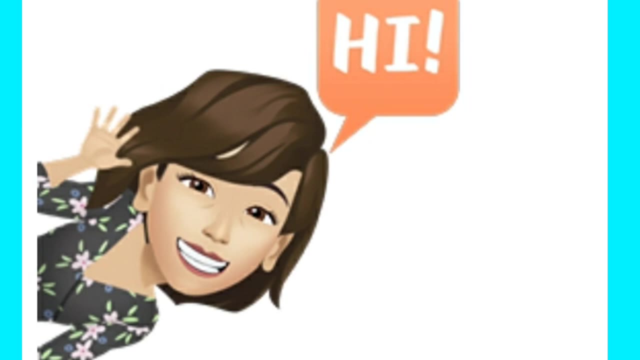 want to invite you to subscribe, If you are my current subscriber. thank you for watching and comment here to say hi and tell us where are you watching from. You could let us know what ideas are new to you or inspire you to practice with your. 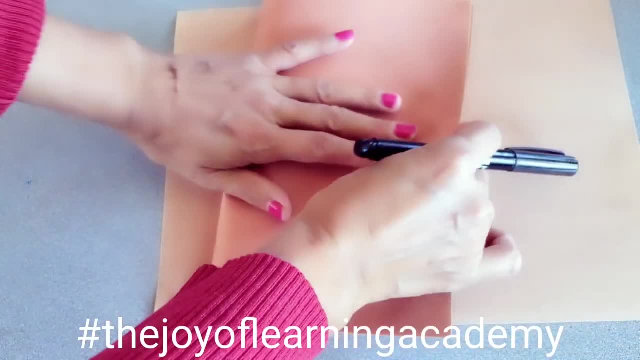 child or student. If you try any of these activities and you hashtag us with the joyoflearningacademy in your social media, you will see the results. that will be very interesting. Thank you so much for watching and until the next videos. See you in the next videos. 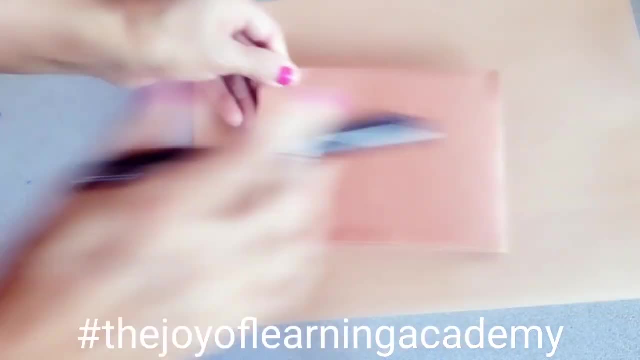 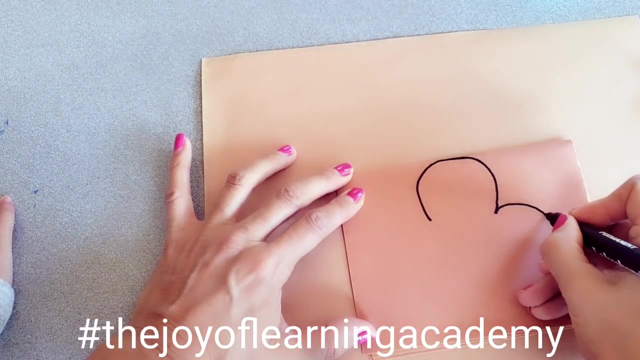 media. we will shout and share your picture in our next videos. Our goal is to inspire you and continue to make a difference in children's lives, extending our community of educators, moms, learners and more. So let's get started. Our first 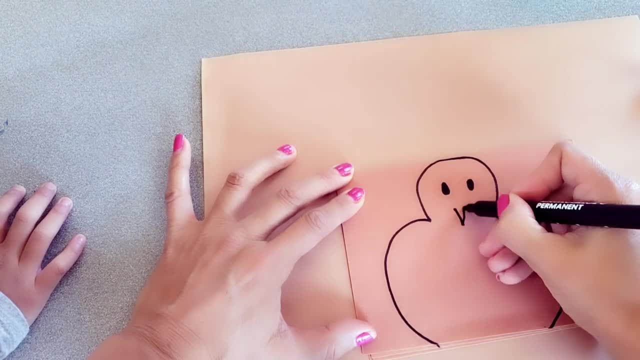 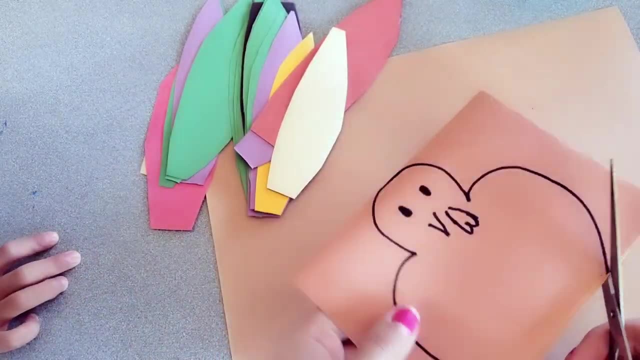 activity will be making turkeys. These turkeys are very easy to make. All you need is construction paper, markers and scissors. You can just draw how I'm doing. then you need to cut it and you also need feathers. It will be easier for me. 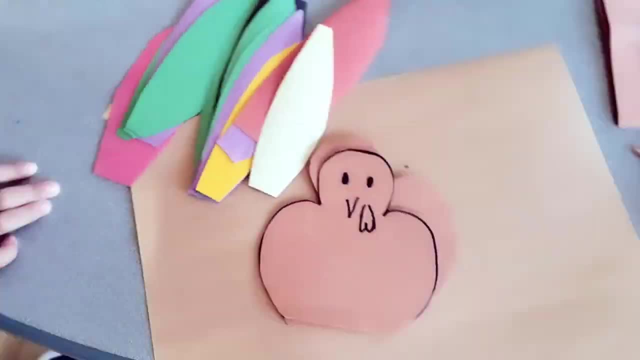 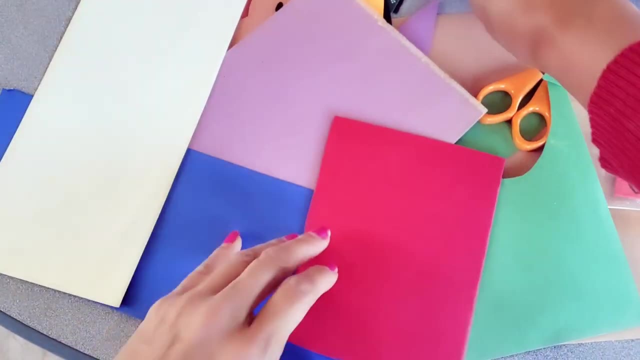 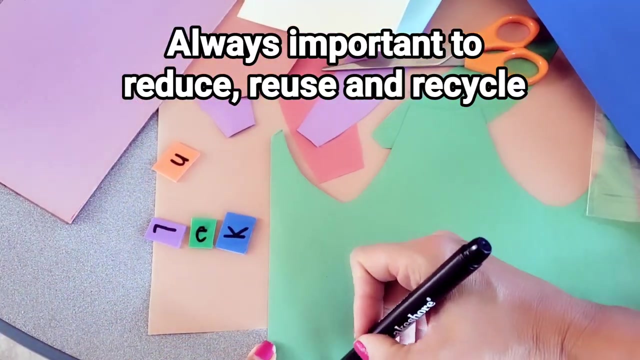 to cut them, and I already have them, as you may see, for younger children. But if you have children ages two and a half, use this activity to help them develop their fine motor skills by having them cut. Remember that the process is more important than the outcome, and you don't want to miss any. 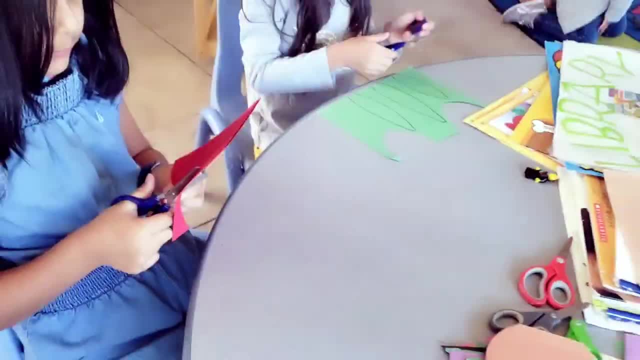 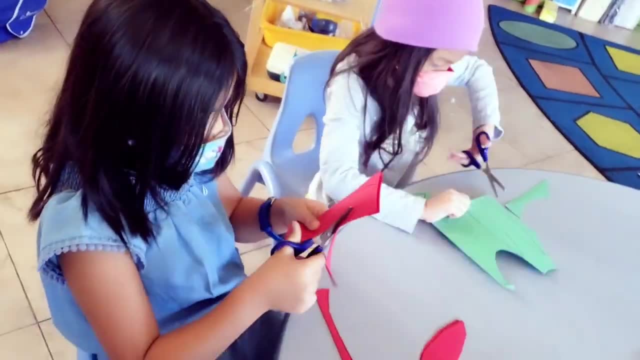 teachable moment To extend the activity. we're using the turkeys. You can use it for your child to learn his or her name. In the past, we also used the feathers for children to tell us what they are thankful for Be. 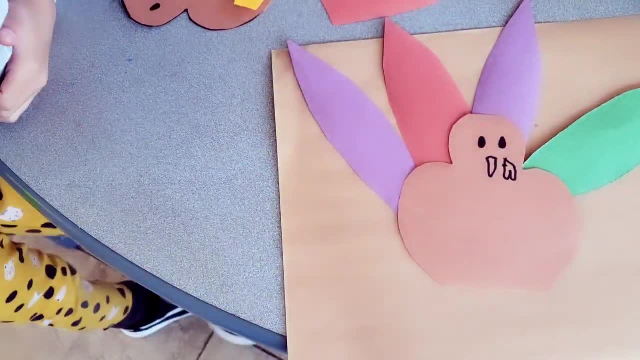 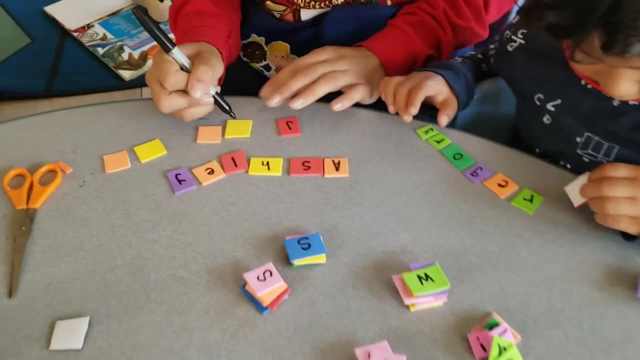 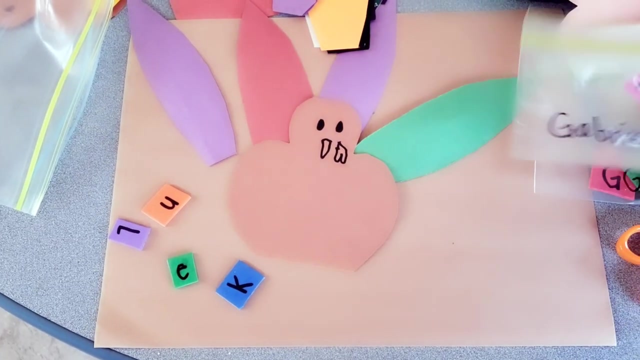 creative and, most important, engage your child and your students in the process. We're also getting letters ready using foam paper for them to make their names. To help younger children be successful, you can separate the letters in a plastic bag, like we are doing, and then just to place it in the right order For older. 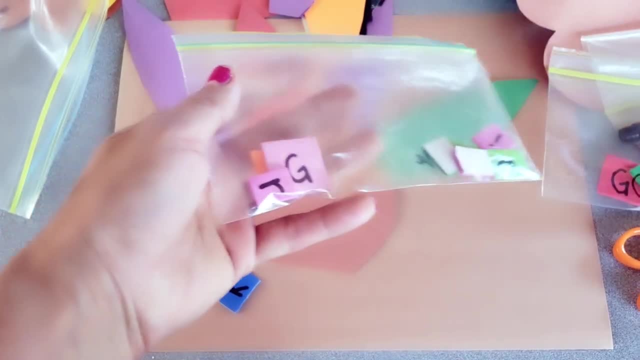 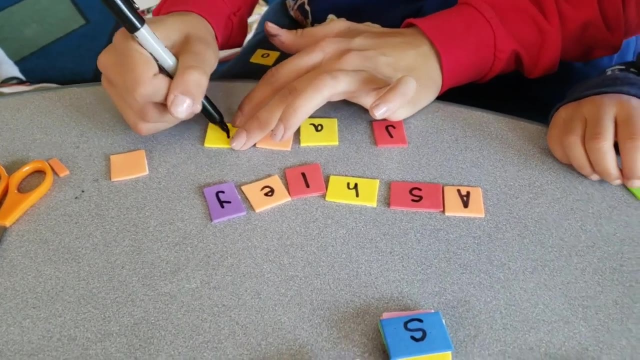 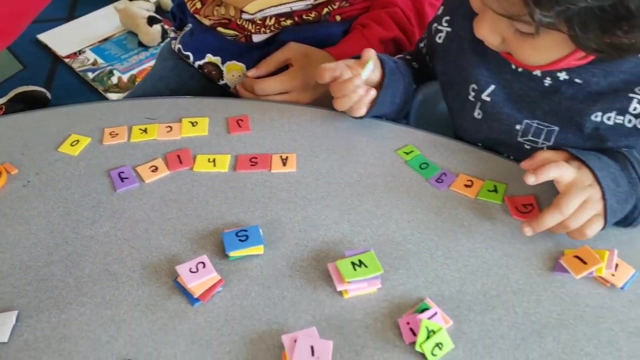 children or children who master their name. you can just have different letters and have them choose the letters they need. Remember we are facilitators and we want children to be successful, so make sure that you adjust activities for your children according to your students' development and challenge them. 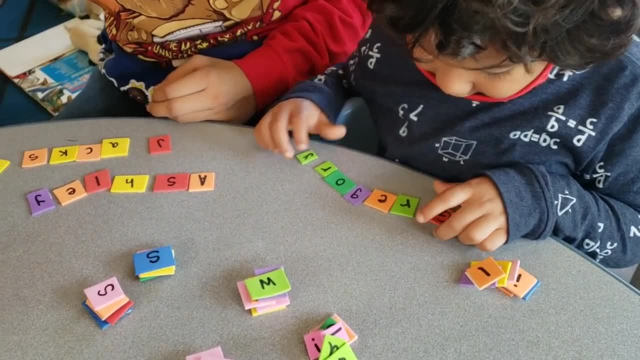 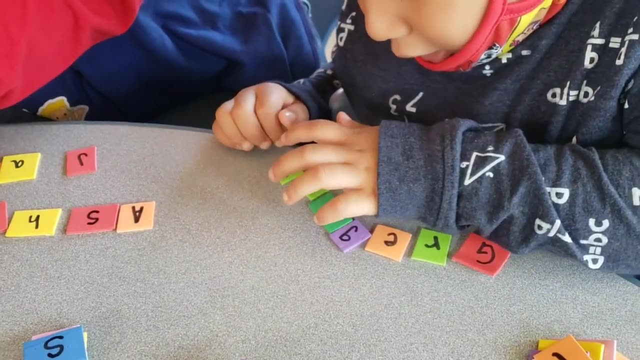 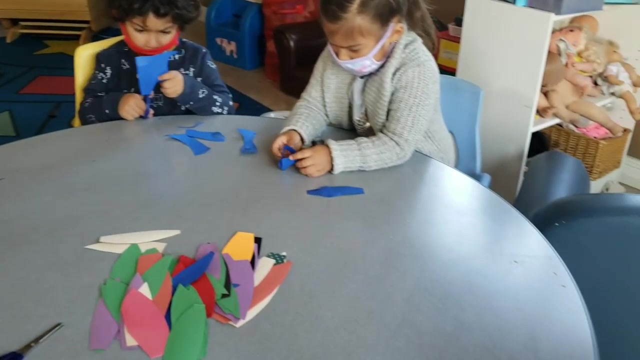 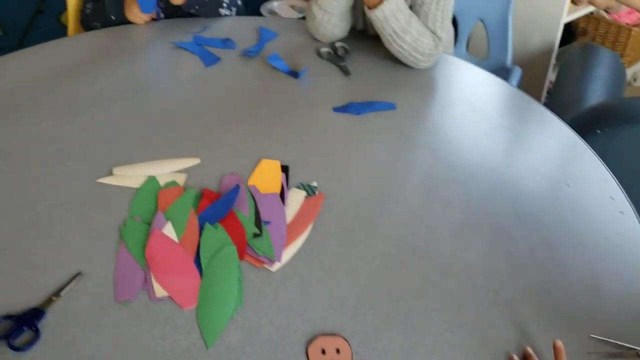 whenever you need them, Give me your name, Gregory. These are mine. These are your letters. Can you tell me your letters? G-R-E-G-O-R-Y? Very good, Yes, Now we have your friends' names here. Okay, I see Matthew's cutting here. He's little getting some help. And then Leilani cut feathers. 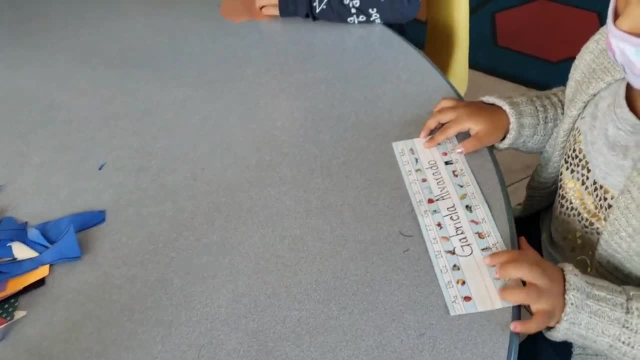 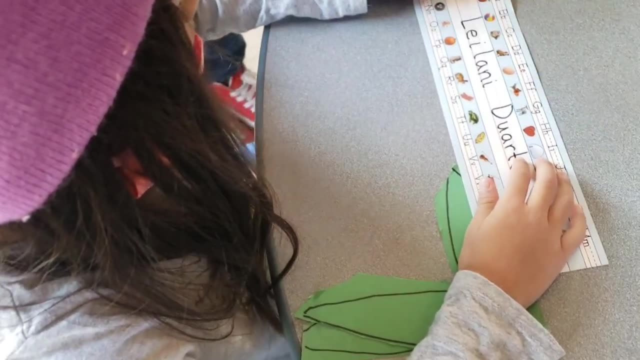 Eight. That means you're going to have your. turkey is going to have. how many feathers? Eight, Eight, Leilani. let's count, Leilani, Count. No. start in here Your letters: One, two, three, four, five. 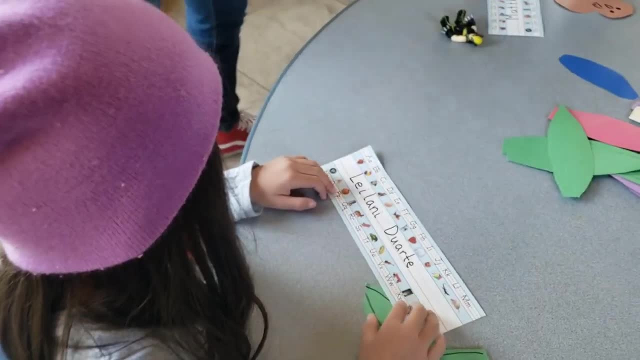 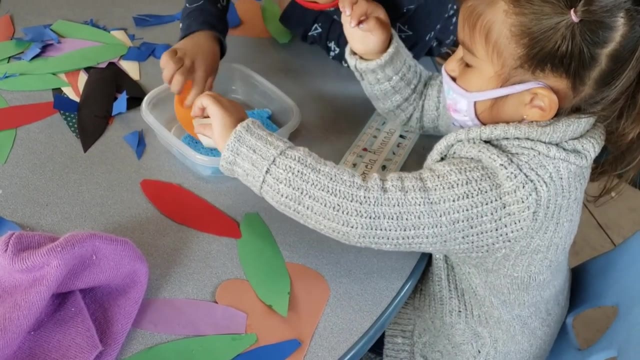 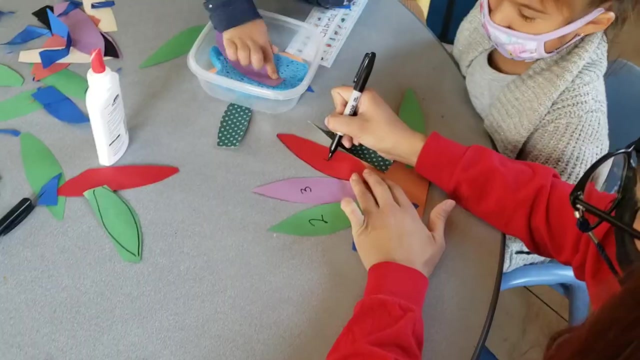 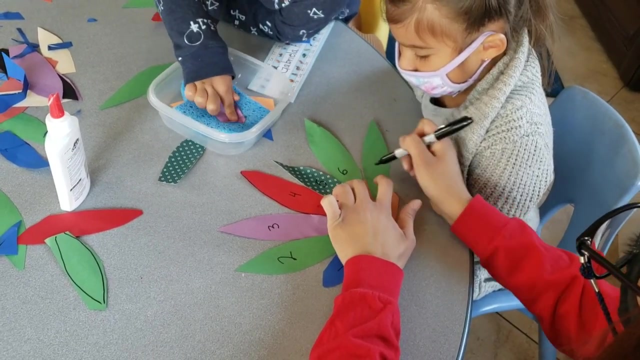 Six, Seven, Seven. So your turkey is going to have seven. Are you done? Are you done? Okay, How many more do you need? I need more because of that turkey And after four, Five, Five, Six, Seven. 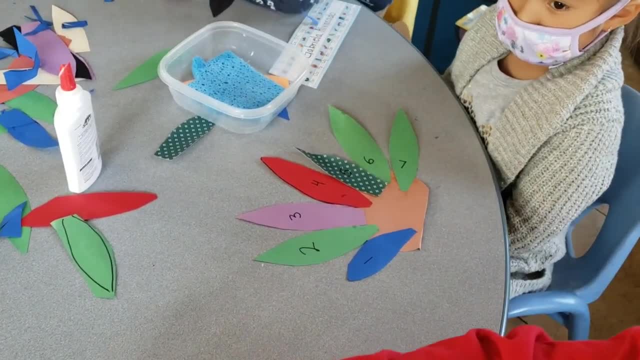 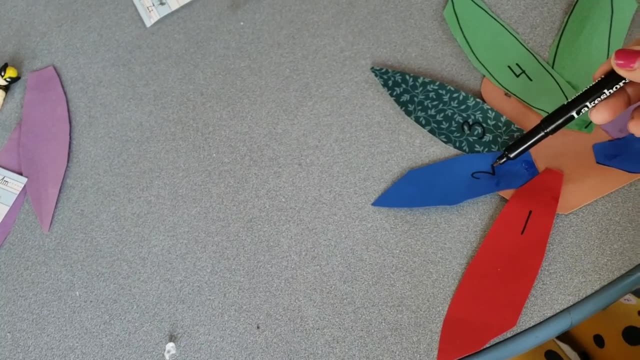 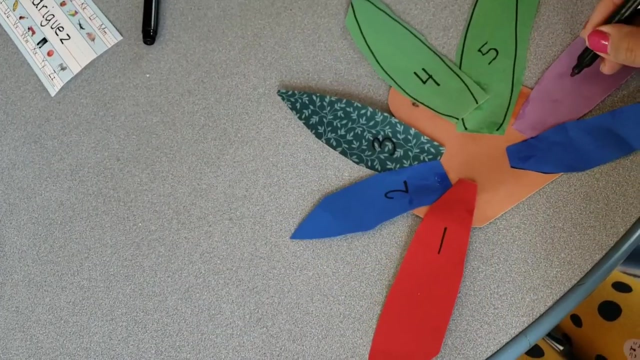 Good job, But your name has eight, so you need one more. feather: One, two, three. Your name has seven letters. Let's count One, two, three, four. What's after four? Five, Five, After five is: 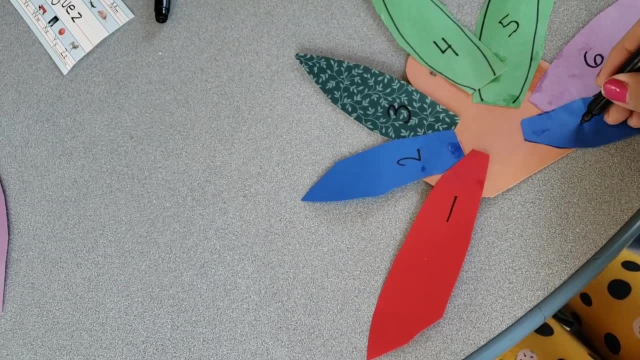 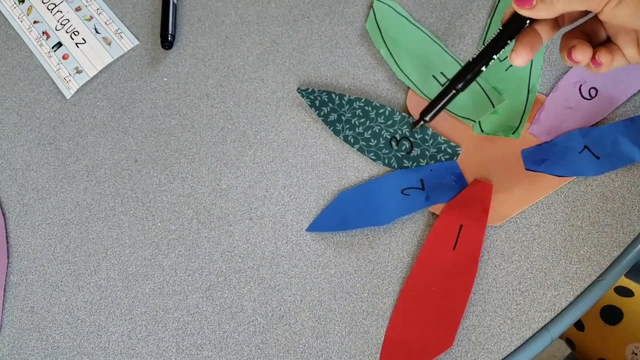 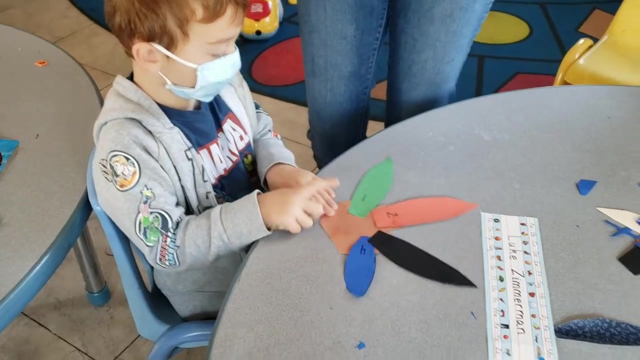 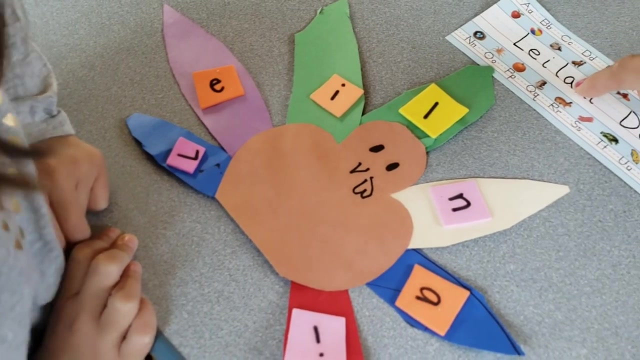 Six And Ten, Seven. Let's practice, because in here we get a little confused. One, two, three, four, five, six, seven, Four, Two, Your names: L, E, I, L. After the L comes: 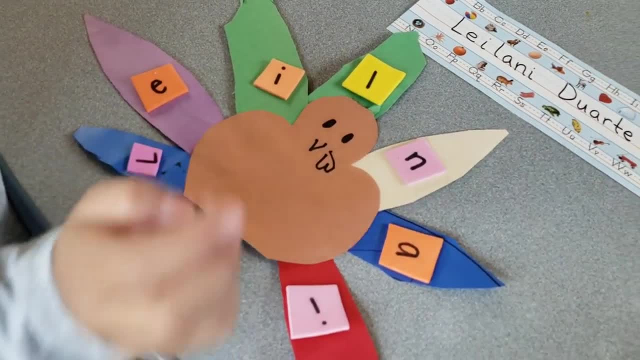 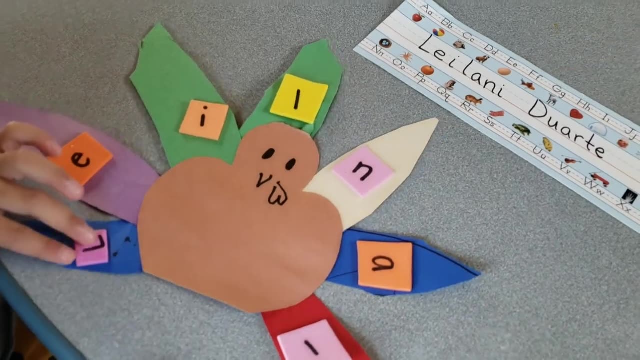 Letter A. Where is the letter A? Solanetel, Solanetel, Aha, Yes, Okay, Now that one is supposed to go after the L. So what are you going to do? Stretch, Okay, Switch. 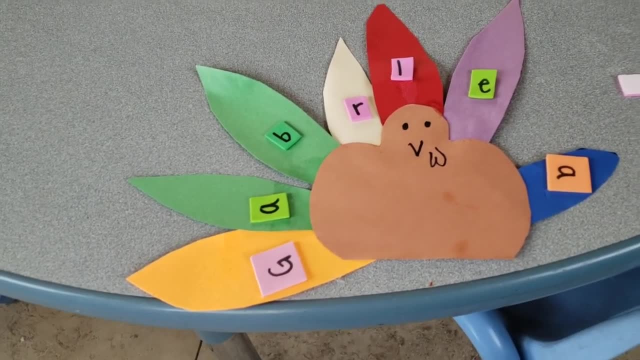 Gabriela. Oh Gabriela, you're missing one feather A times the letter C. Is that what you have? Are you peeling? I know it's a little hard. You did it. You're peeling the sticker. Now you need to pull. 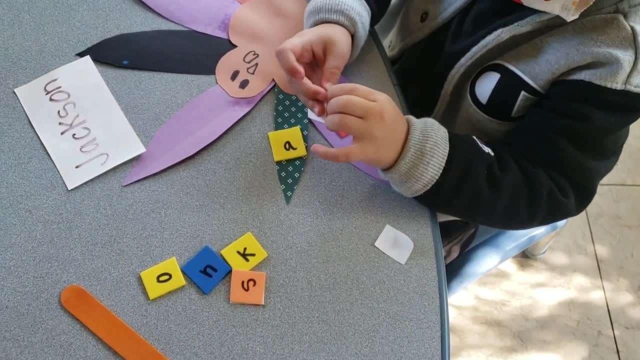 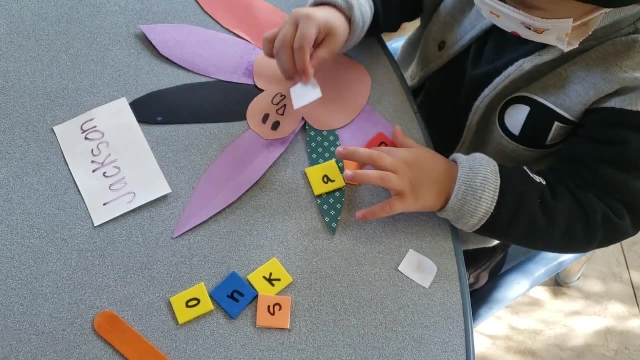 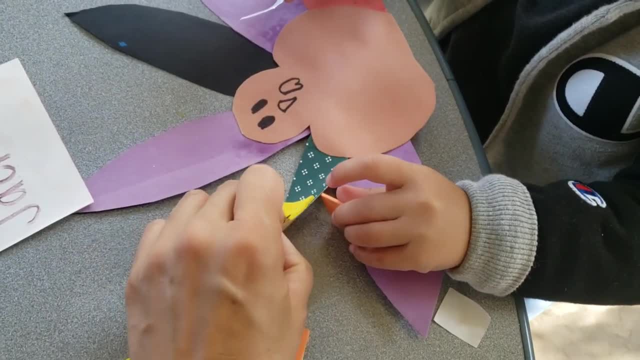 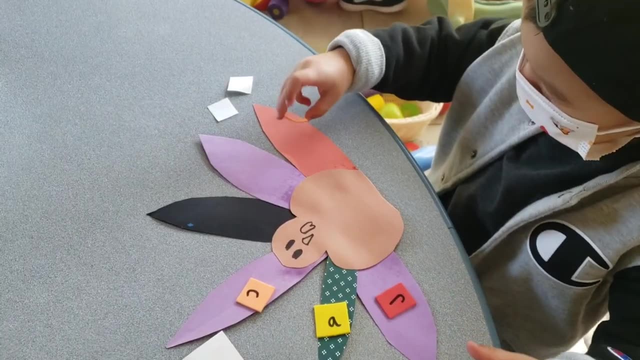 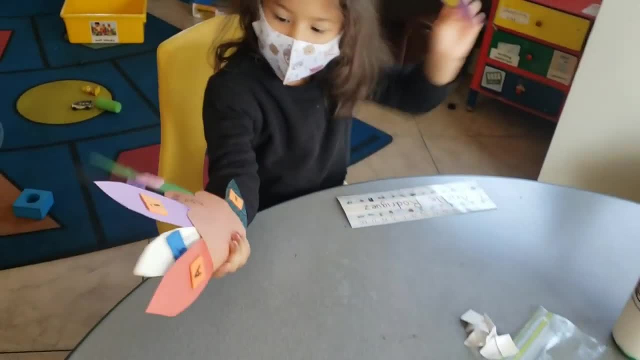 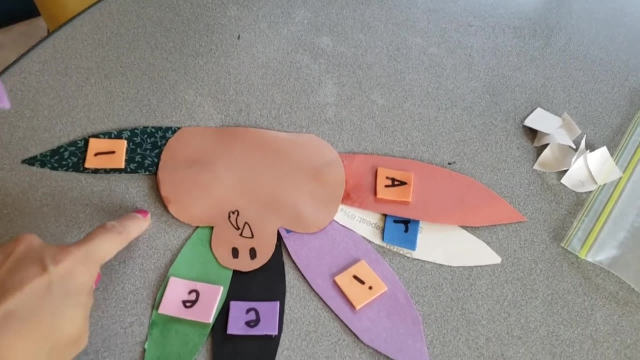 You did the letters. May I see the letters if you match? Ariel, Oh, you need the letters, Okay. Okay, let's switch it up. On which leaf It's broken Where? What happened? Typing, Typing. 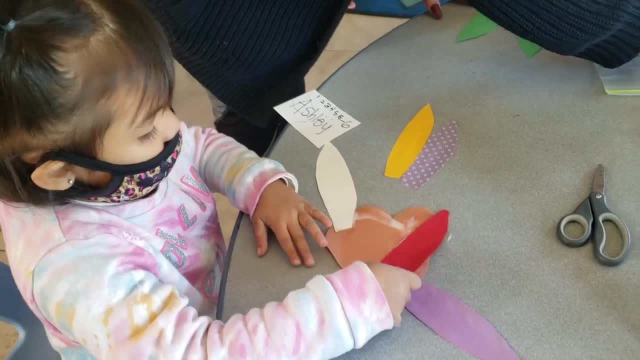 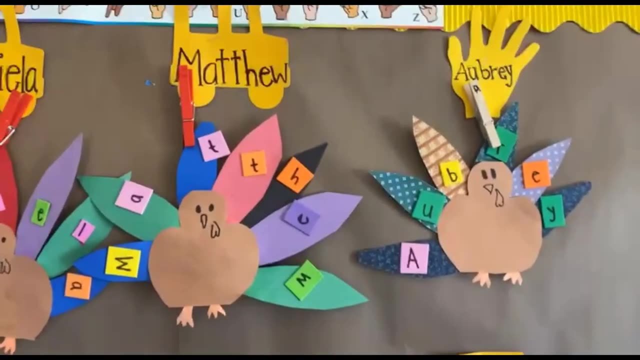 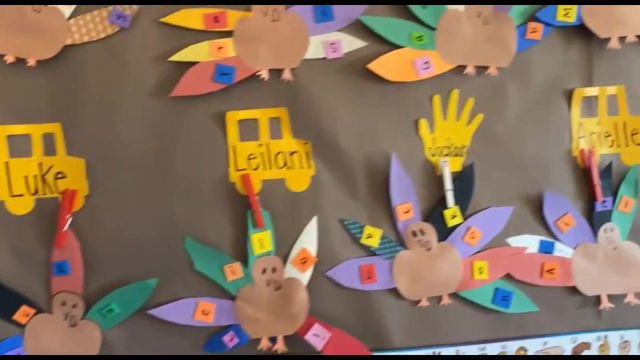 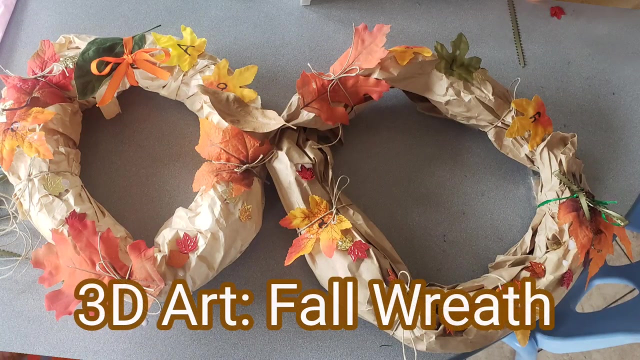 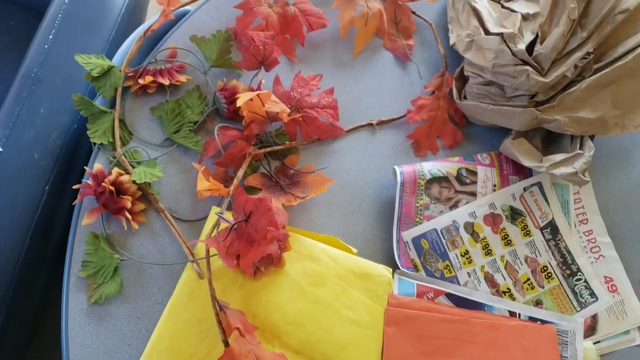 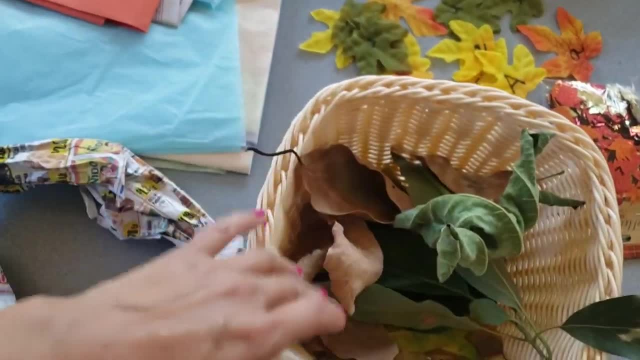 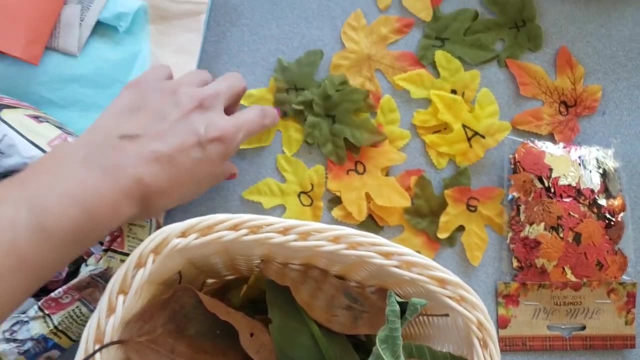 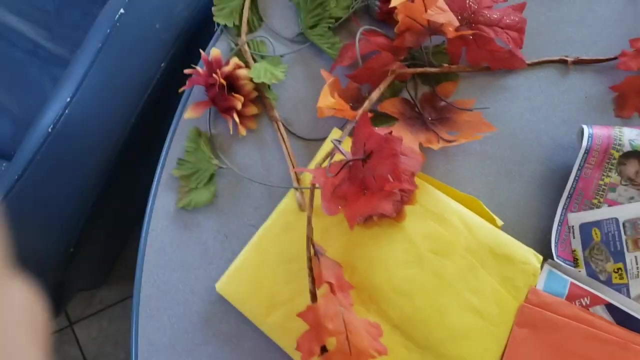 that you have at home. I have here leaves, dry leaves, that kids could put on here to decorate, or we have shiny ones, and then we have these leaves that we were using for name matching, and then I have some of these leaves in here. I'm gonna use some scrap paper that I have and, if you have, 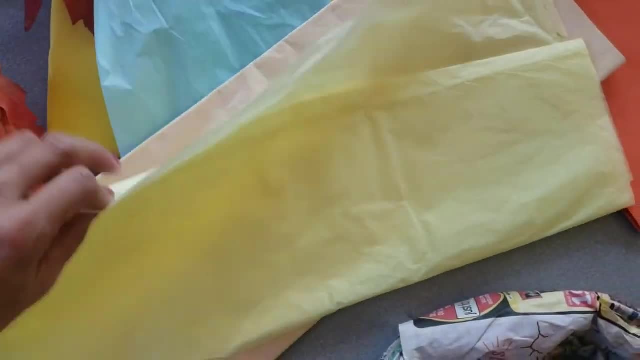 tissue paper that is orange or brown. that would be even nicer, but these are the tissue papers that I have, and then I'm gonna put this on here, and then I'm gonna put this on here, and then I'm gonna put, And then you need some tape. that's all you need. 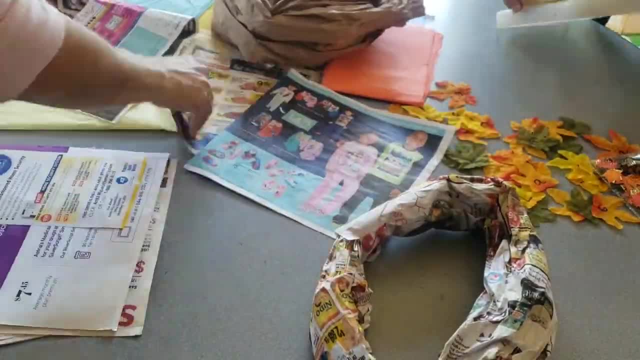 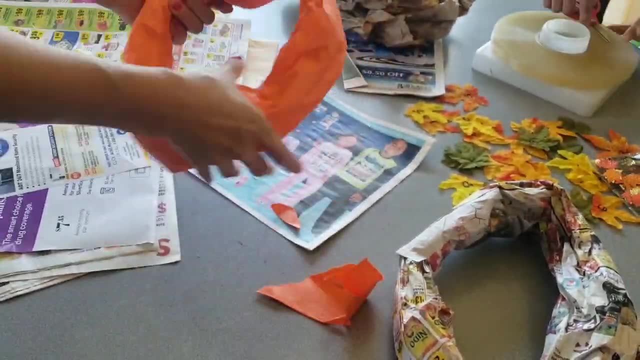 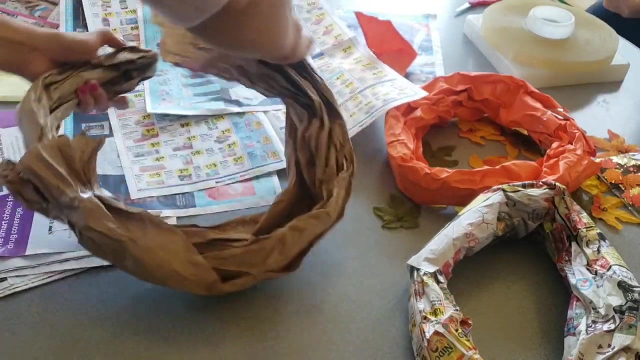 So you have to make them. it's very simple. all you have to do is squish paper, and I'm trying to make different styles of using different kind of papers. I'm using some thick paper, so you could have an idea. Not all our work has to look the same, and that's what I always try to emphasize, because 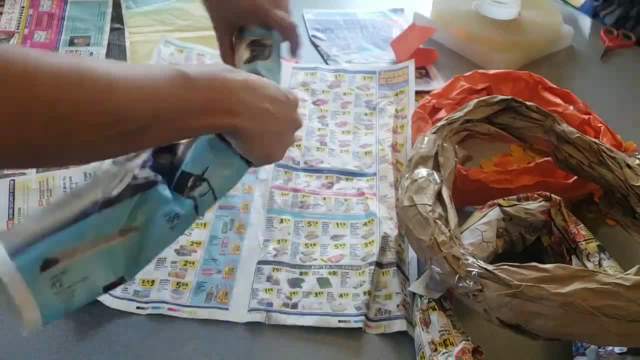 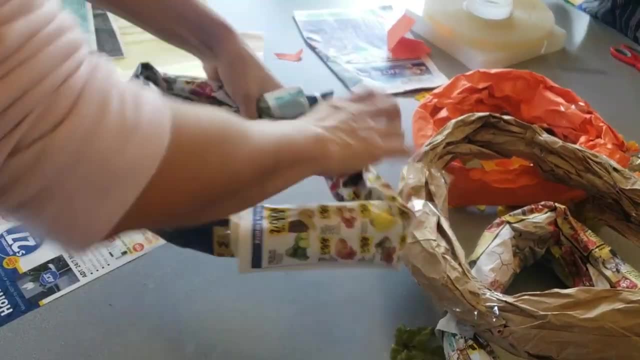 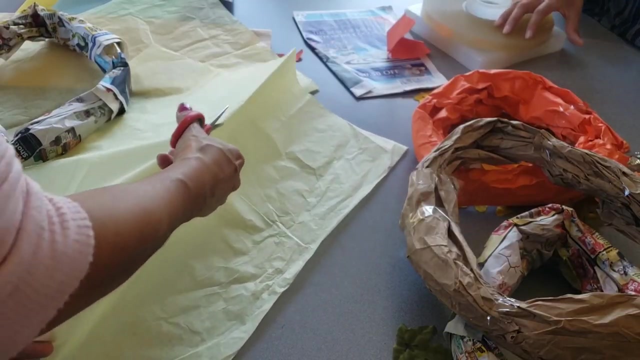 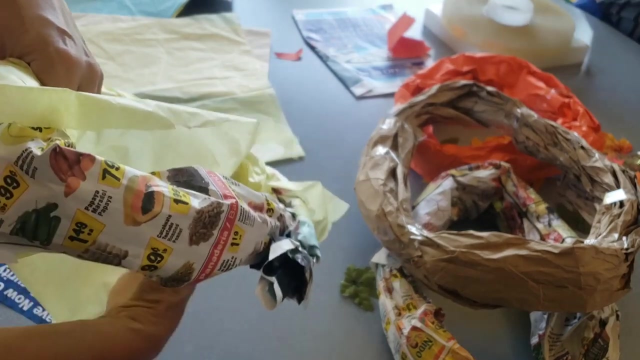 not all kids work need to look the same. I like when our students create their own masterpiece, because each child is individual and unique and I like to allow and have room for them to create their artwork as a unique piece of work. It is extra work to do this, but it's all worth it, because then at the end of the day, they 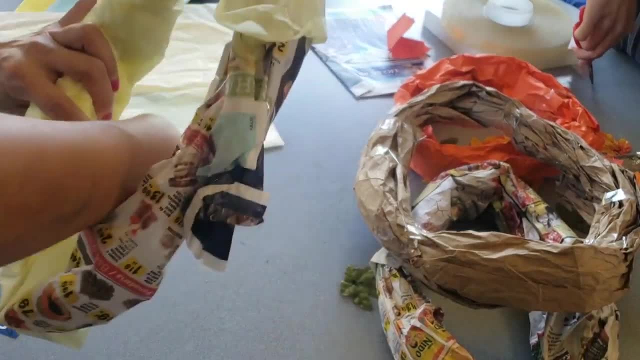 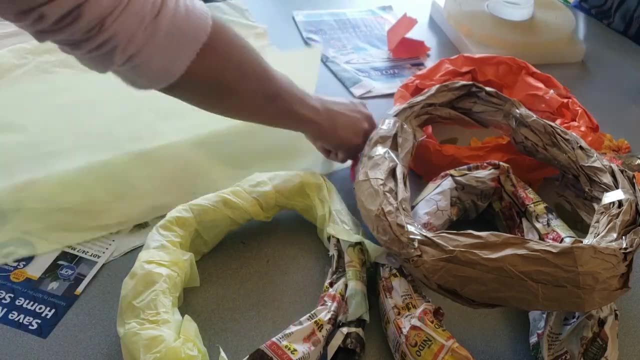 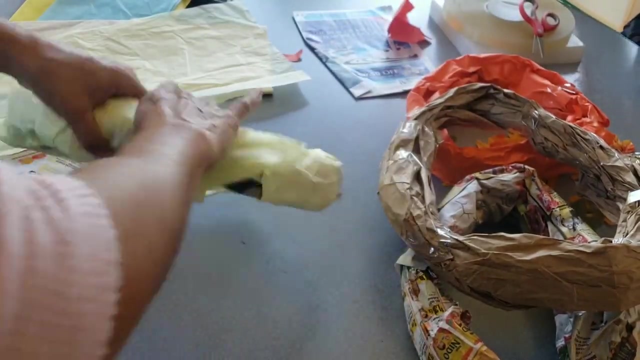 have their own unique piece, as they are unique. So here I am. I'm using tissue paper for some, so students could have many choices when they get to choose which one they want to use for theirs. So, like I say, if you have orange tissue or red tissue, paper will look even better. but 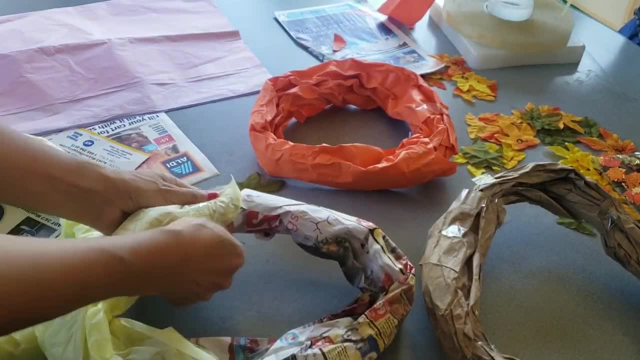 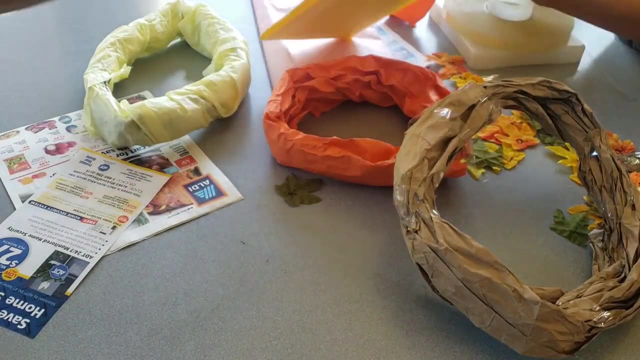 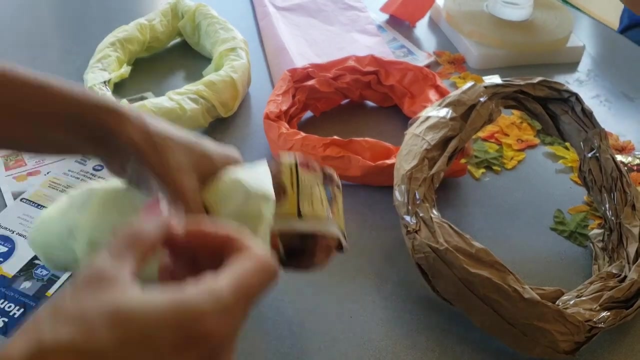 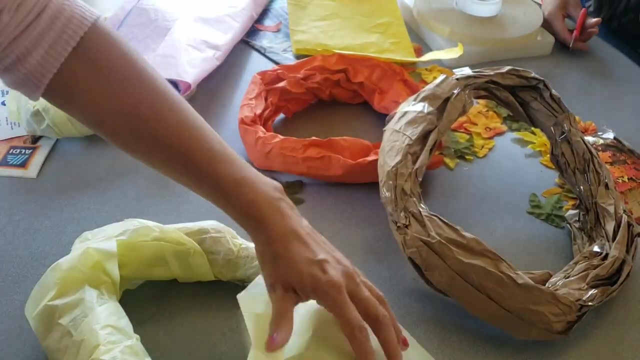 I'm using what I have and I want our students also to see to be resourceful, not to be limited of just one way of doing things. There's many different ways to do things and I'm right now demonstrating how you could use different kinds of materials to make it work and make their riff. 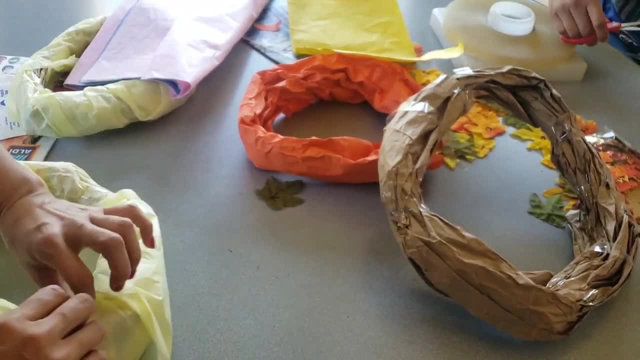 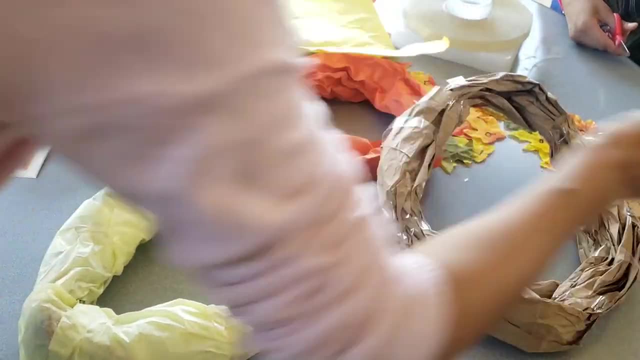 Some of those brown papers you usually get in boxes and we save it because when we get deliveries we get the brown paper. And now I'm going to have my students here helping us because we want to have wrinkles. We want the newspapers to be brown. So I'm going to have my students here helping us because we want to have wrinkles. We want the newspapers to be brown, So I'm going to have my students here helping us because we want to have wrinkles. So I'm going to have my students here helping us because we want the newspapers to be brown. 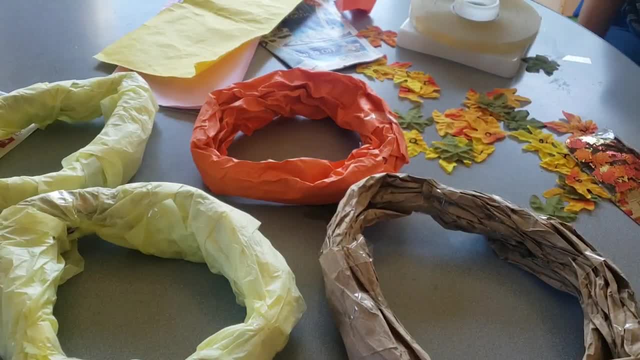 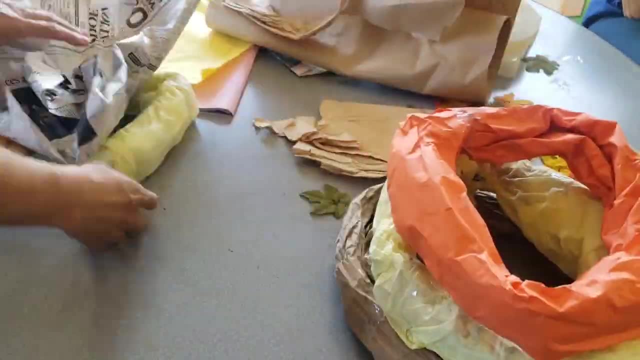 So this is another way to show them about reusing, reducing recycling, As we want to practice that through the whole year, not just on Earth Day. Thank you, Matthew. Now we're going to turn this wrinkled paper into something beautiful. 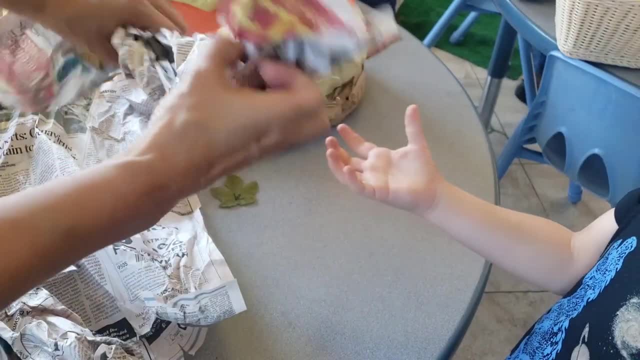 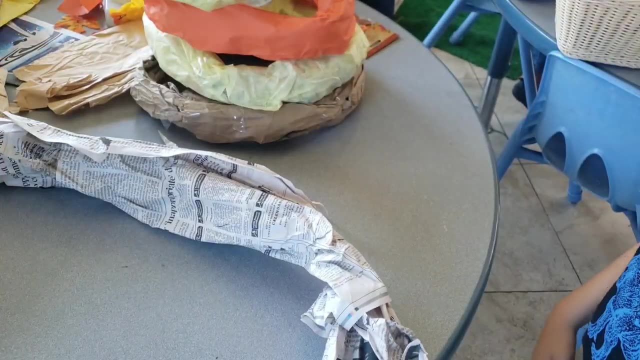 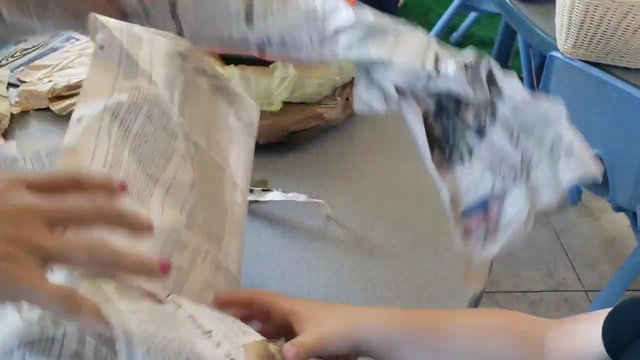 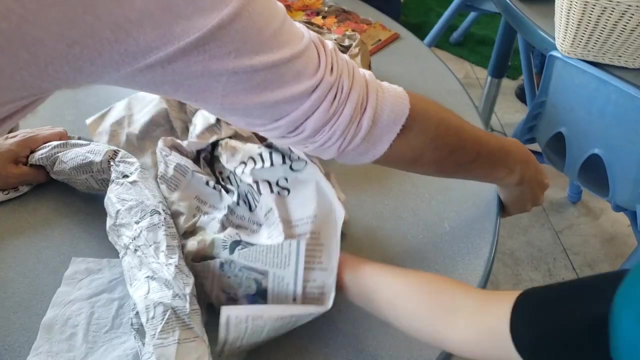 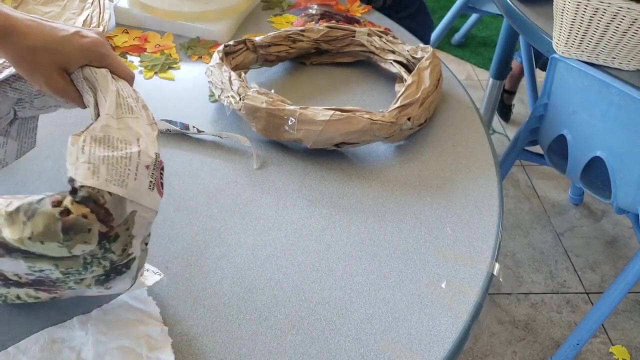 Thank you. Now these wrinkled papers are going to be wrapped up like this: Can you wrinkle this paper? As a teacher, as a family daycare provider? moms, caregivers, we have to be able to multitask, and don't forget to have pleasant conversations with your kids that are around. 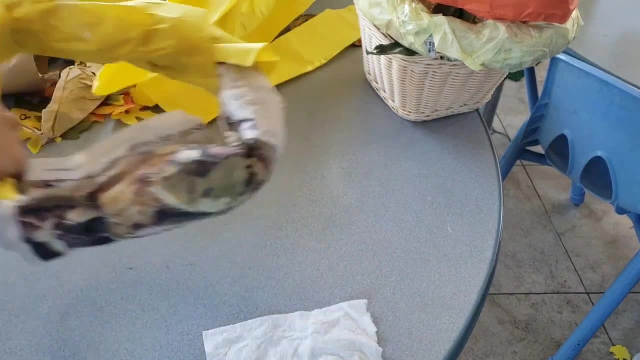 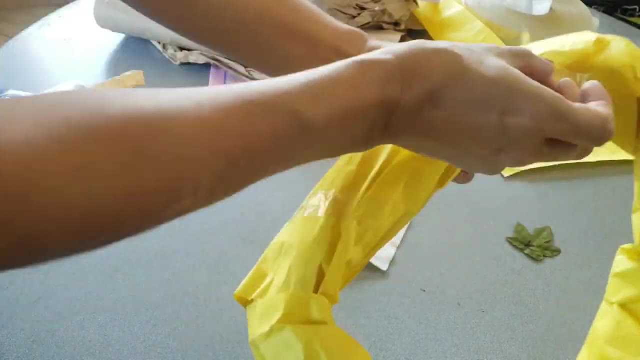 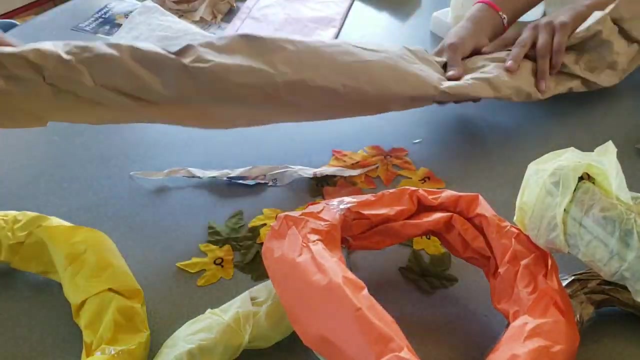 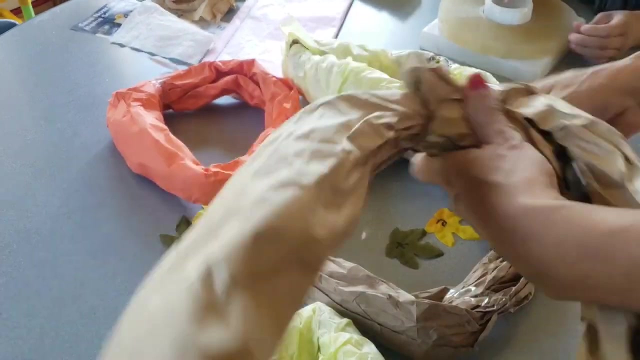 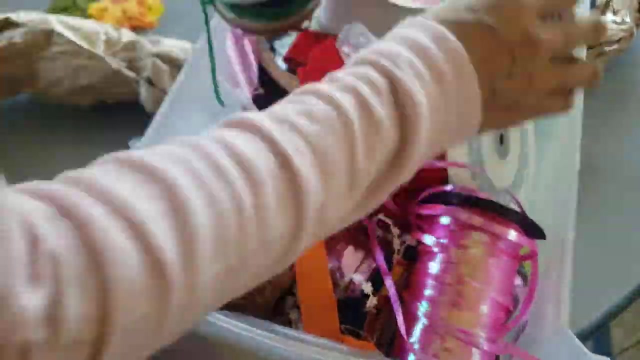 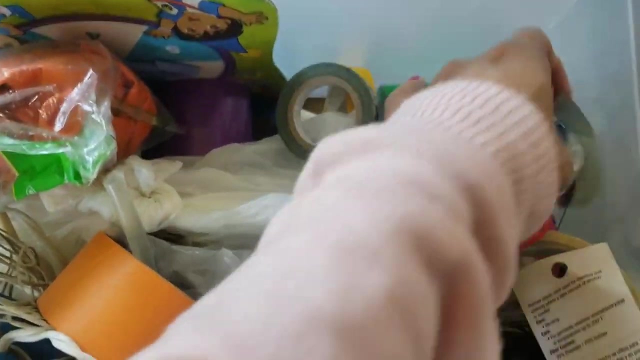 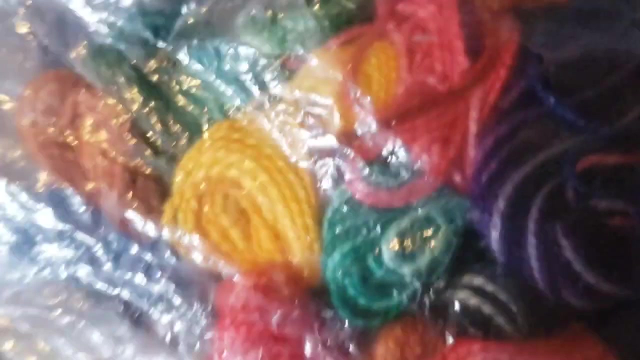 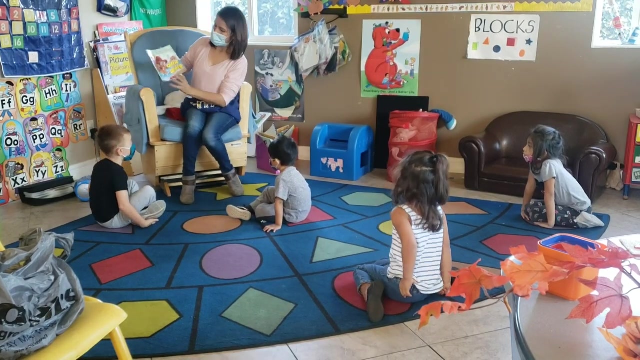 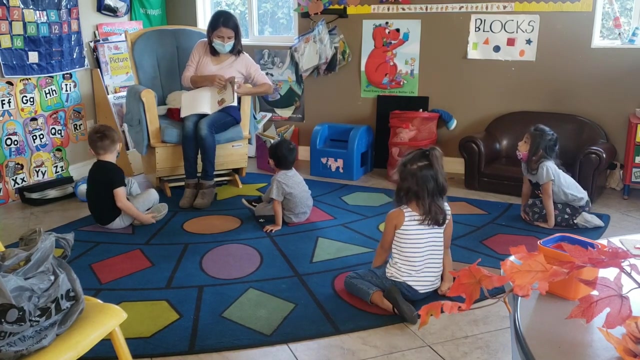 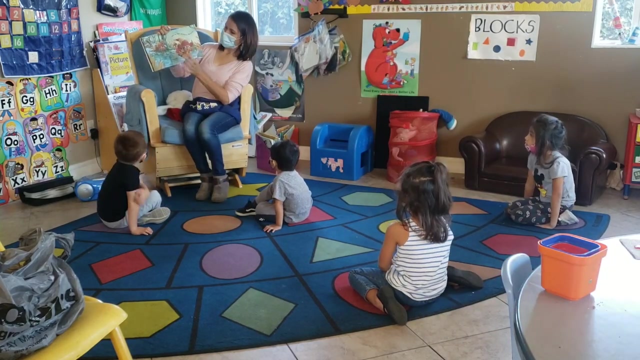 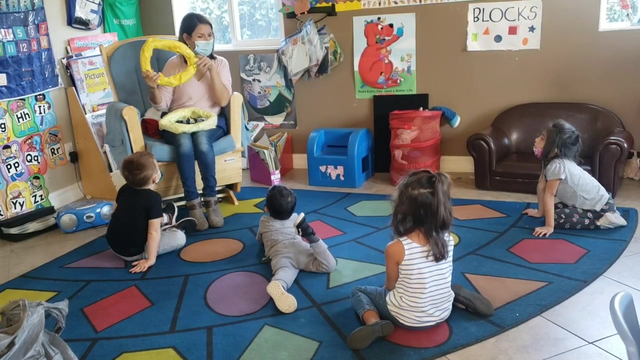 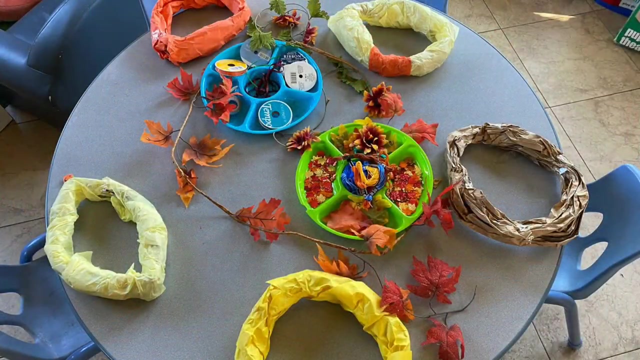 Thank you. Thank you, This is a song. It's actually a song. It has the notes of the song: What we're going to do in this shape. what's the shape? Circle, Circle. We put it different colors. Some of them are light yellow, some of them are like this. 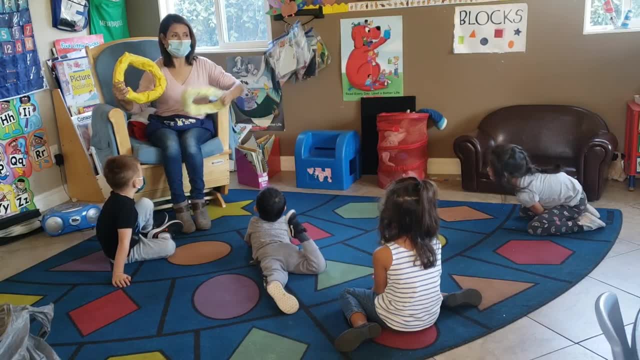 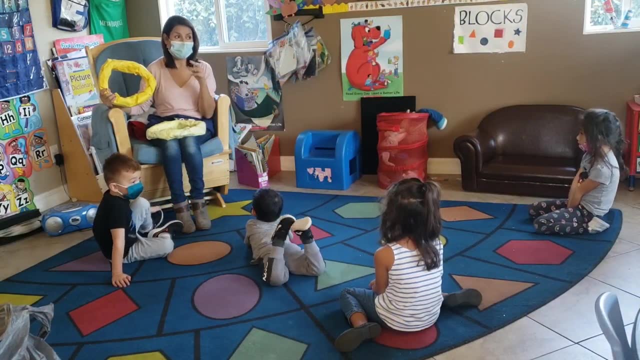 You guys have to be careful, because this one has tissue paper and it could break. You guys are going to decorate with whatever you want. We have leaves, we have ribbons. we have tiny little leaves that are like kind of like shiny. We have bigger leaves, however you want. 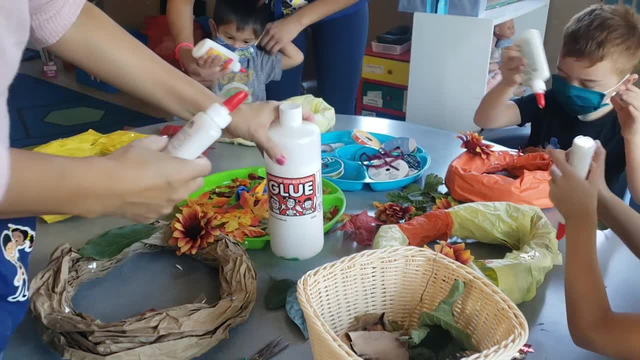 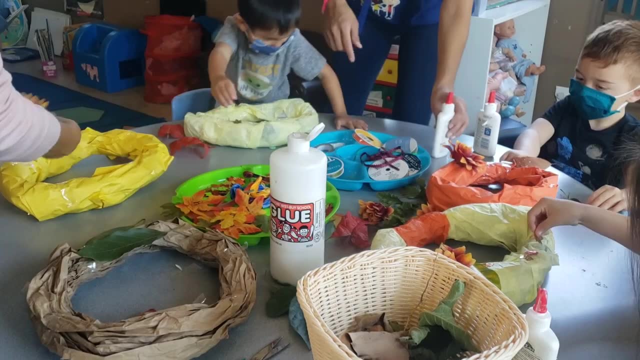 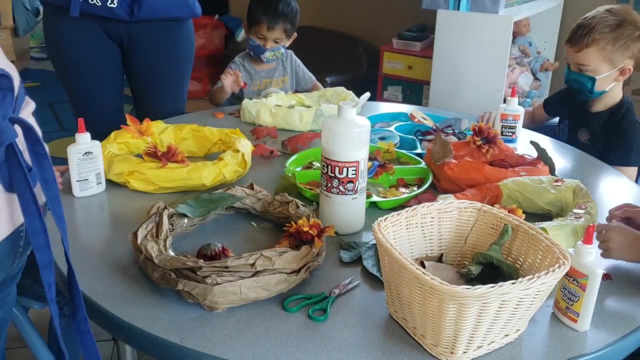 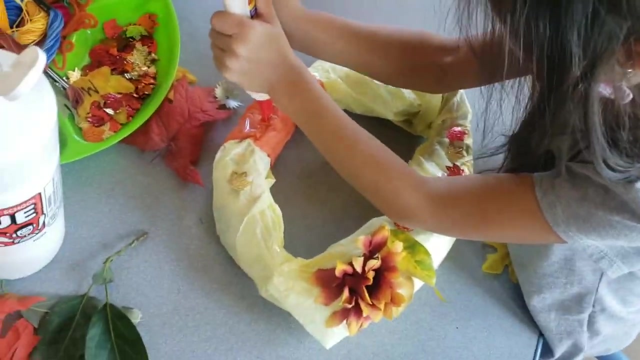 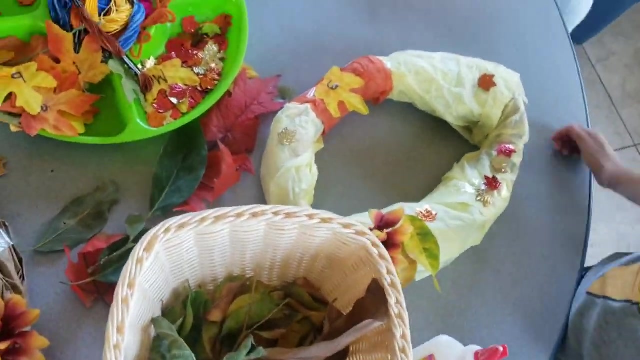 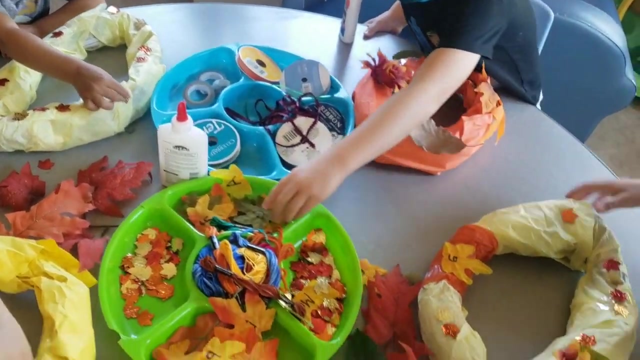 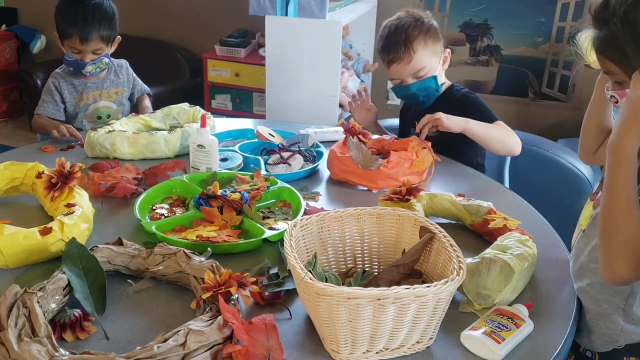 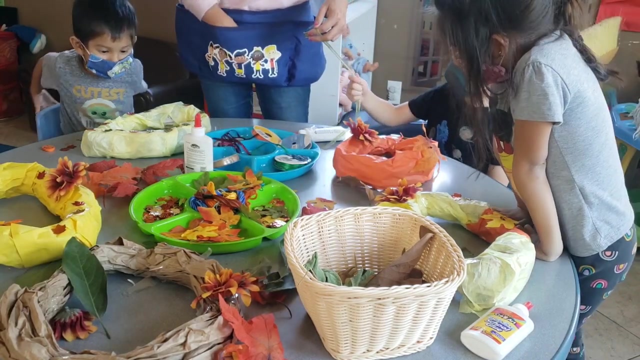 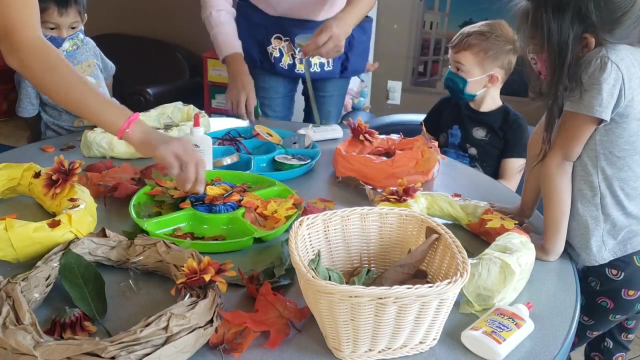 Are you ready? Are you ready, honey, If there's somebody in this room, let me know. Uh-oh, Uh-oh, Uh-oh, You want me to pull this? you want you can pull this side, these big ones? okay, let's. 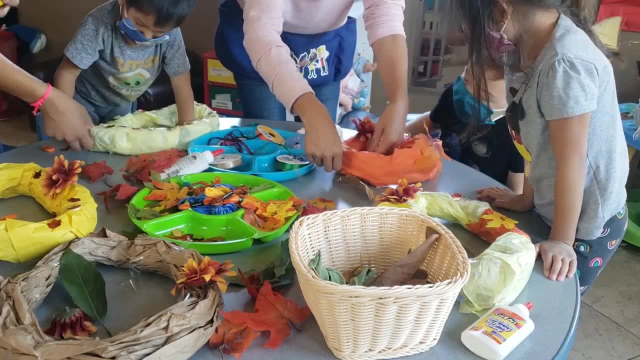 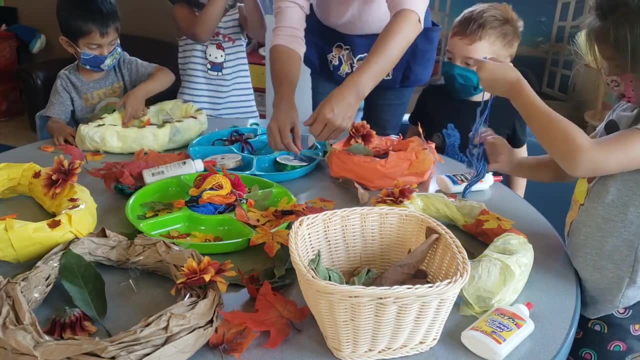 cut. So I'm going to take a knife, hit him in the head. Okay, cut, All right, Let's do that. Okay, So I'm going to cut it. So let's do that, All right, So I'm going to cut it. 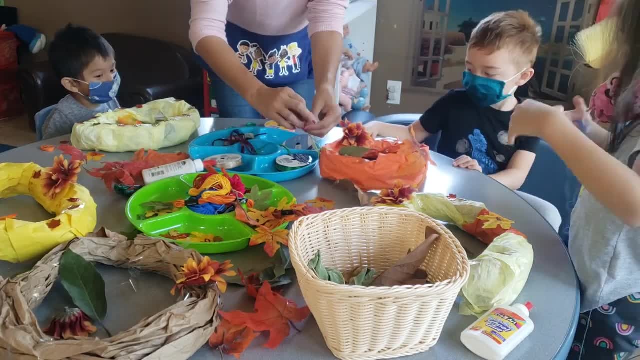 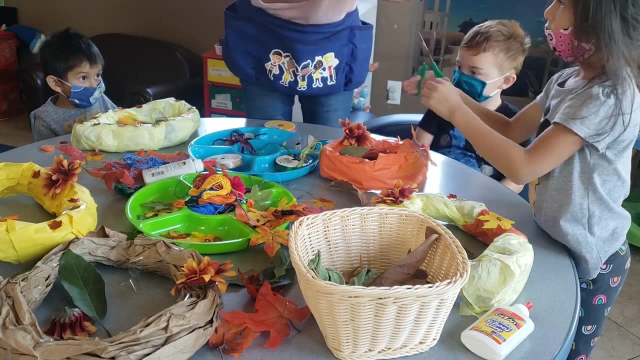 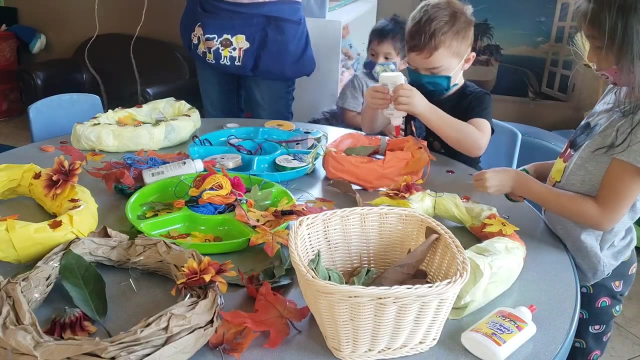 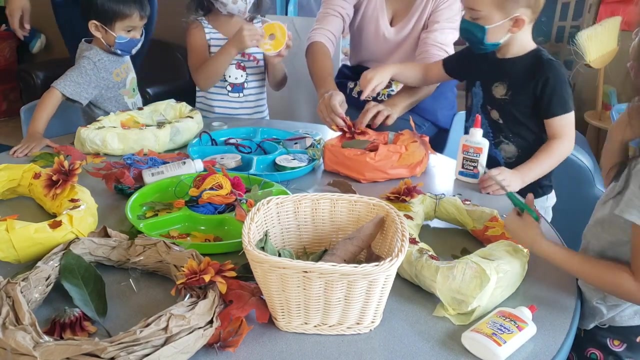 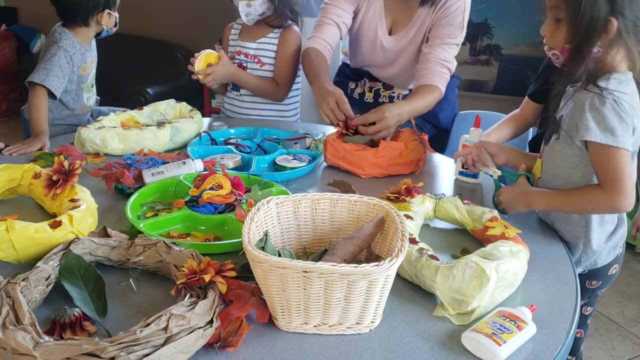 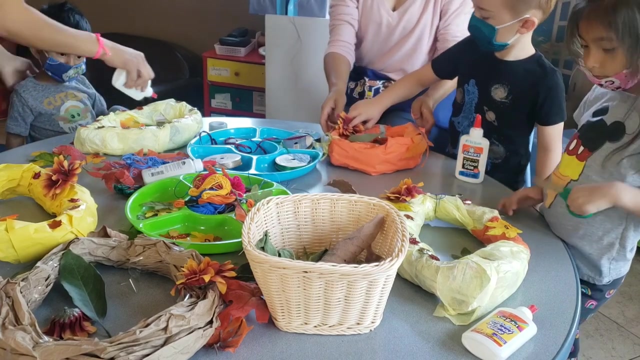 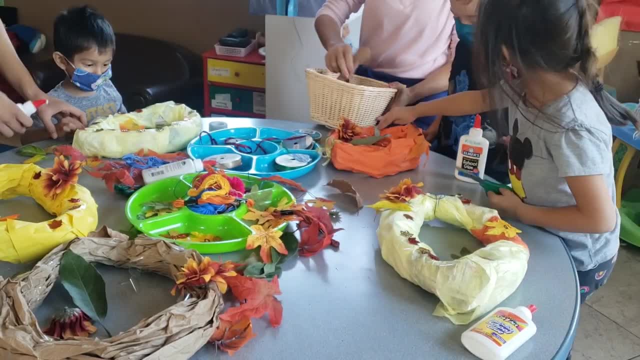 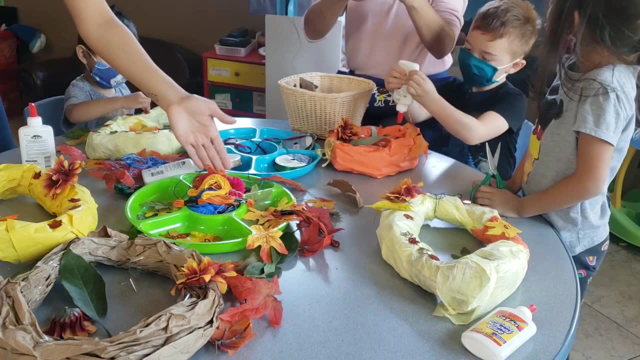 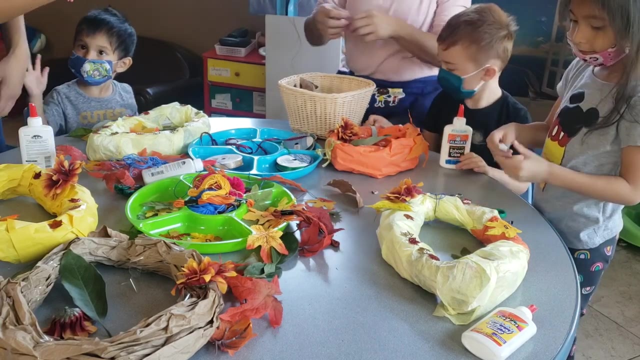 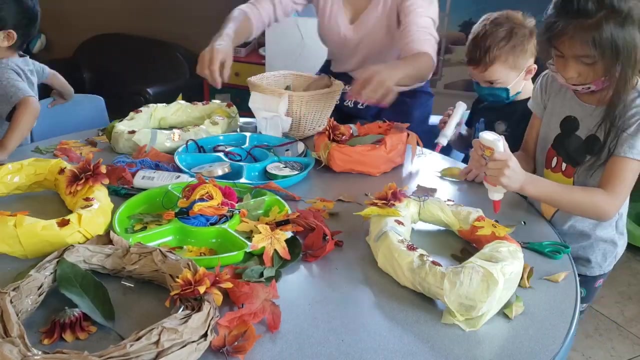 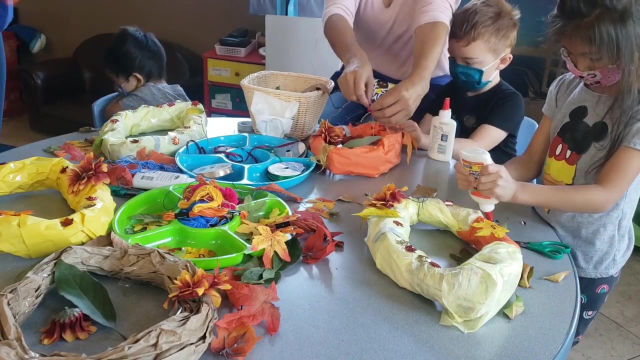 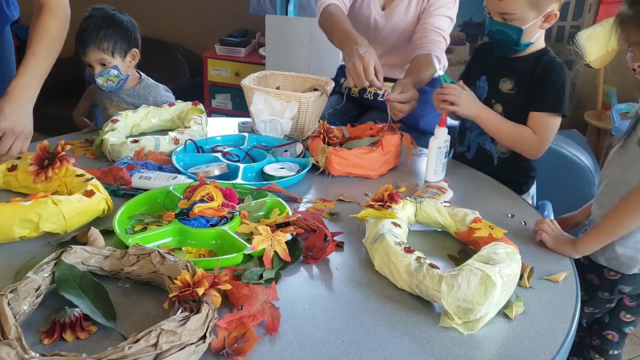 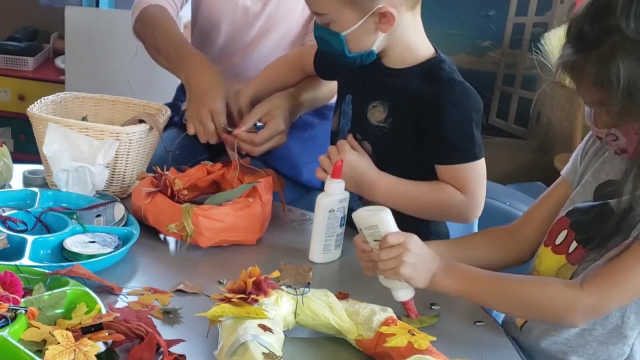 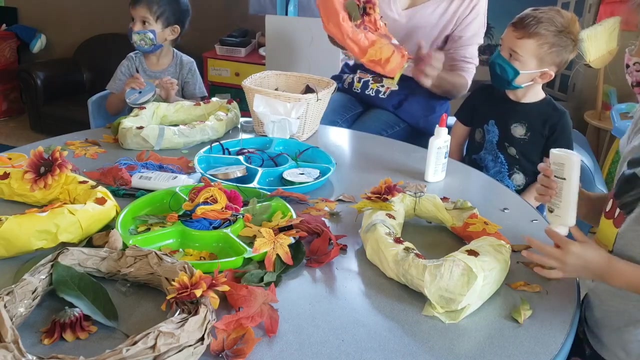 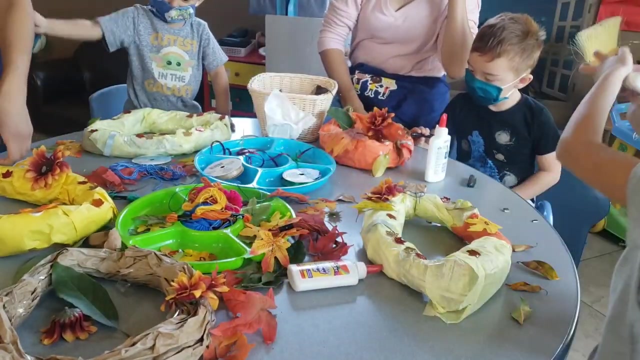 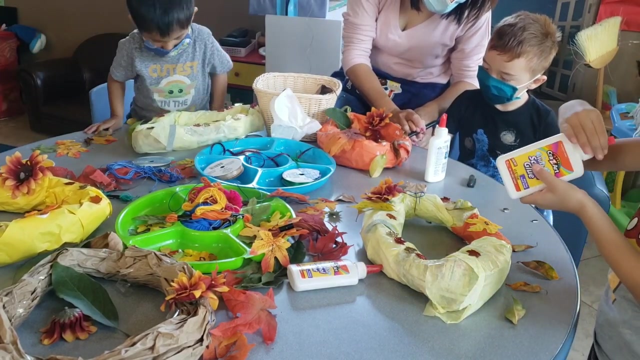 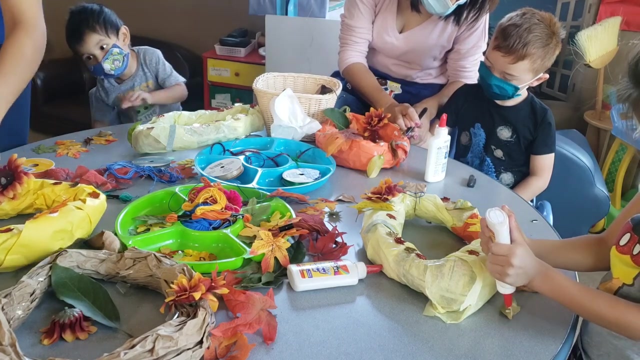 We'll see you next time. Bye-bye L down and here. Look, now you have to do the U? U. That's good L? L. Now you go U? U. The? U goes like this: 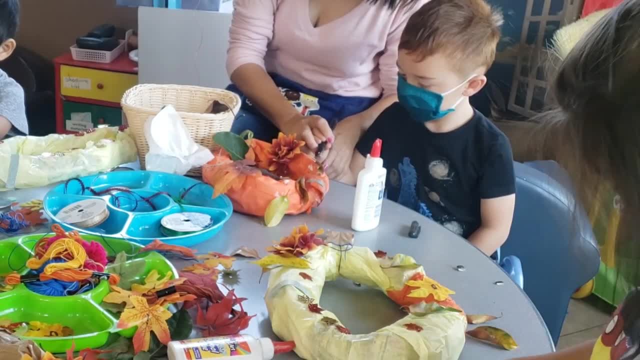 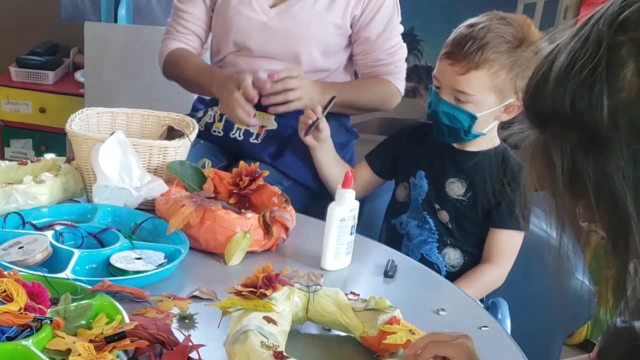 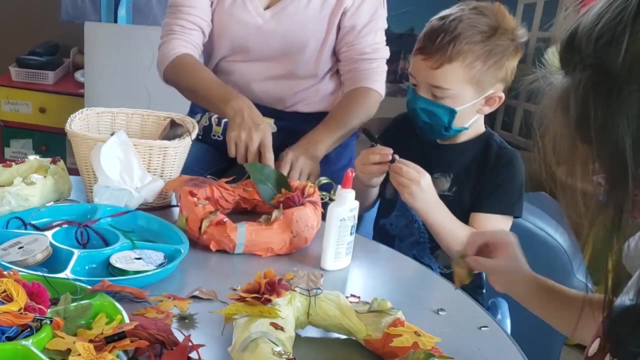 Doon: Okay, Start here. Look Now the K K E. There you go. You want? Do you draw anything here or no, I don't know. Put the link please. I think you have a space to put something else. 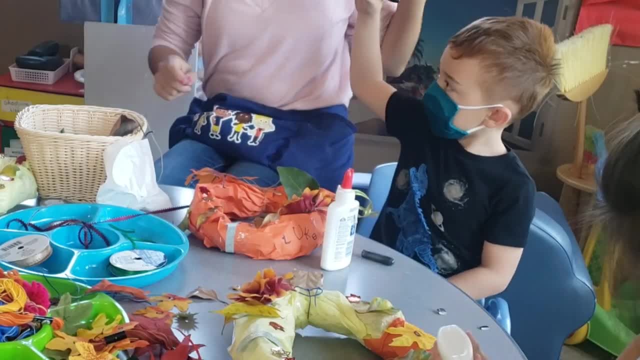 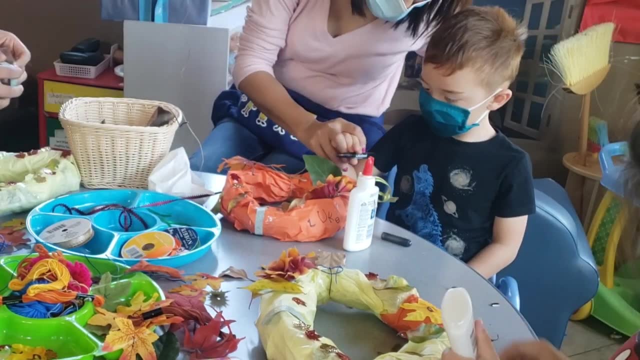 Would you like to get a string or something? You want to draw one. You want to draw one. Okay, you do it. You practice Now. L U K U K And U L U K. 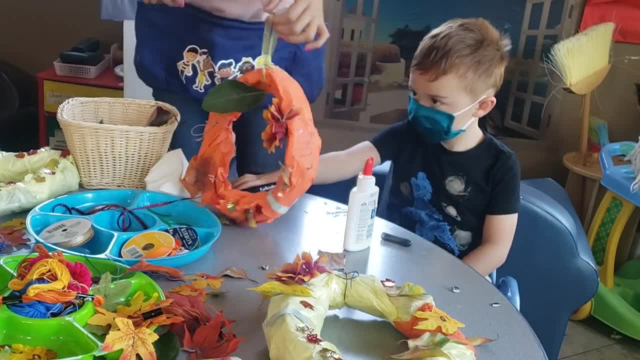 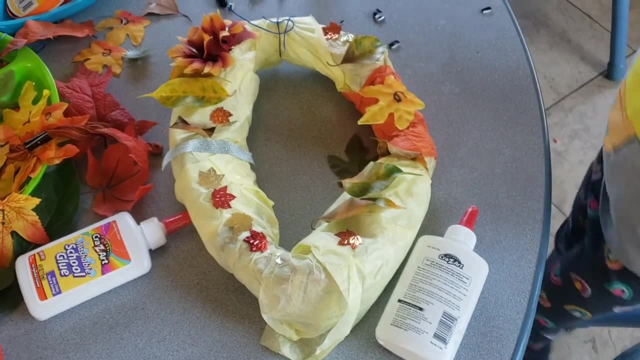 E, Okay, I like it. It looks so beautiful. Would you like to add some more things? I know It's so colorful, Leilani. What else are you going to do? I'm going to take some leaves again. 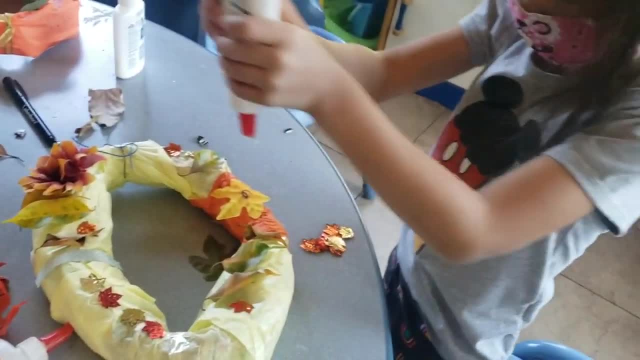 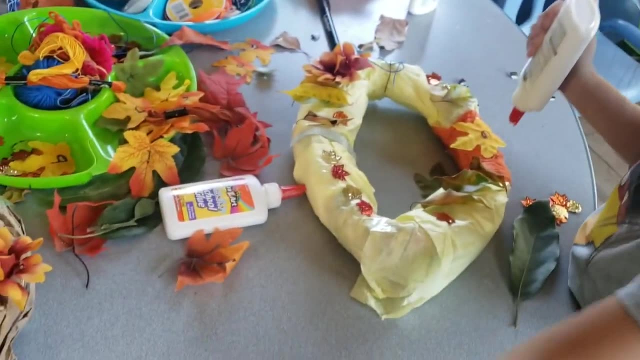 Shiny. Yes, I have this one. If you want, look Dry leaf. That dry leaf is big and beautiful. I have this one And I have this one too. Thank you, You're welcome. Whoa, This is beautiful. 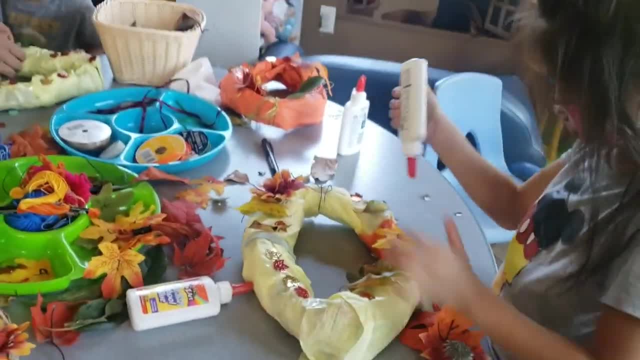 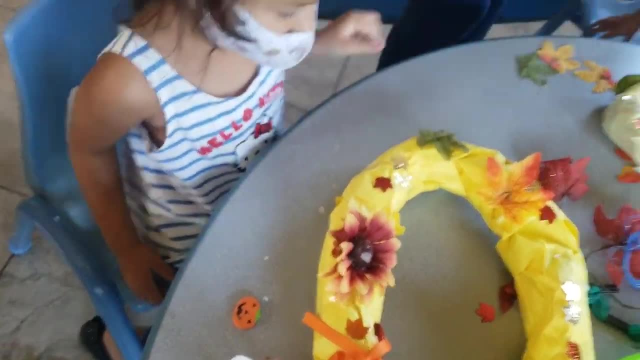 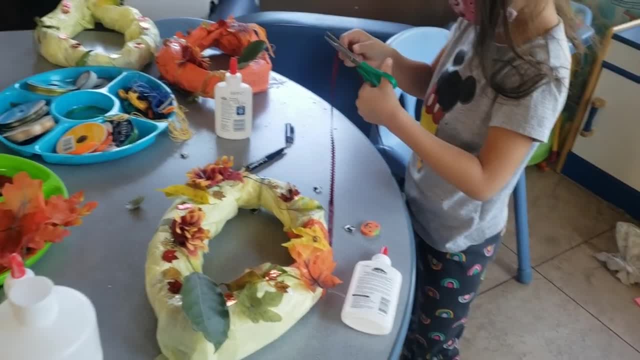 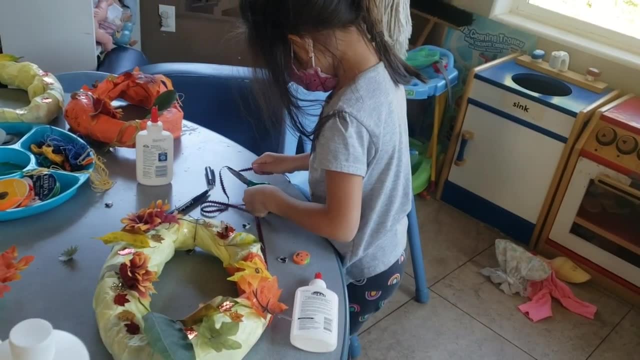 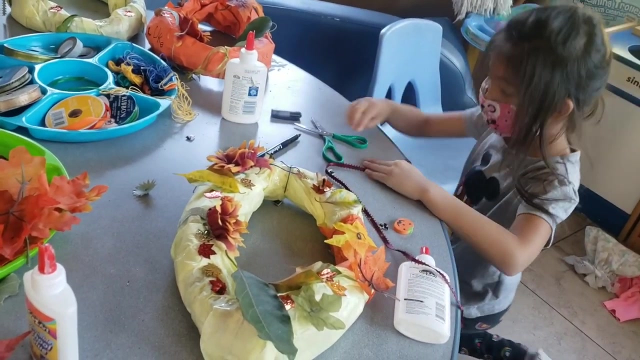 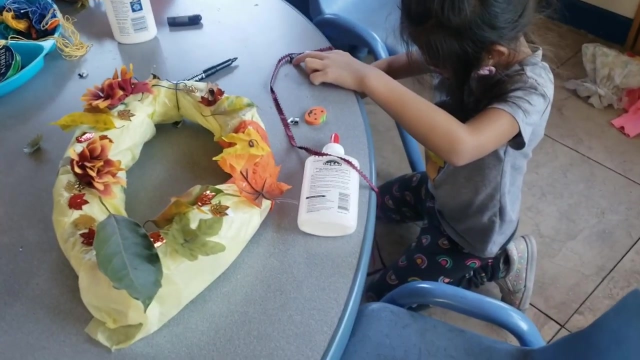 I like it. I like it, It's nice, It's nice. I like it, It's nice, It's nice. Yeah, Keep trying, keep trying. You could do it, Leilani, Don't give up. You want me to help you Holden. 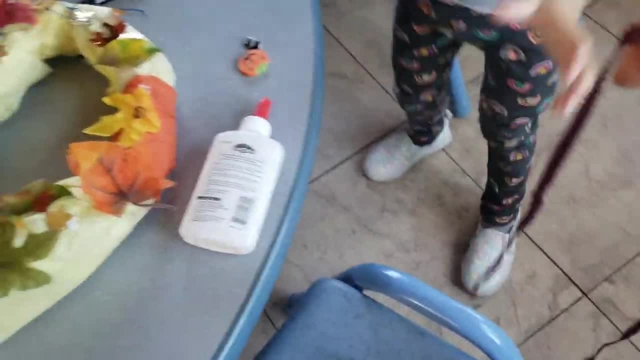 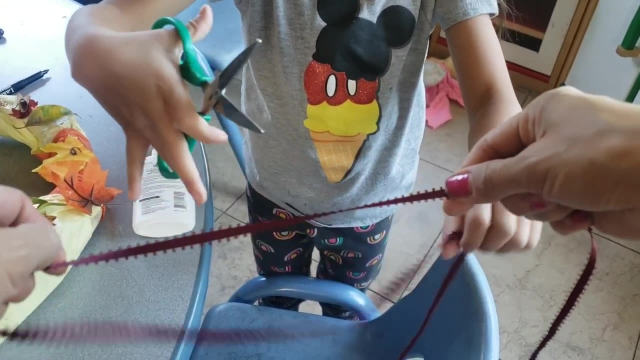 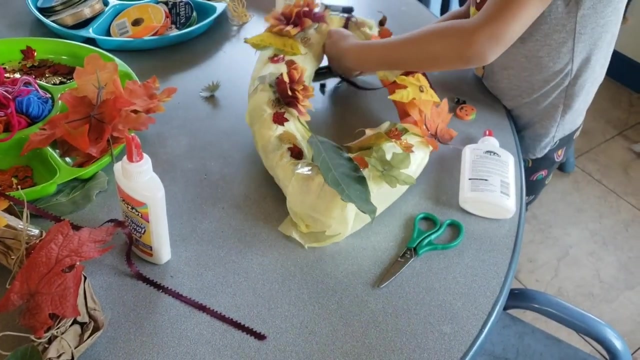 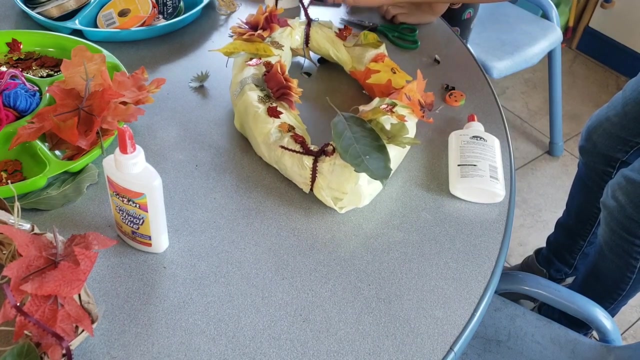 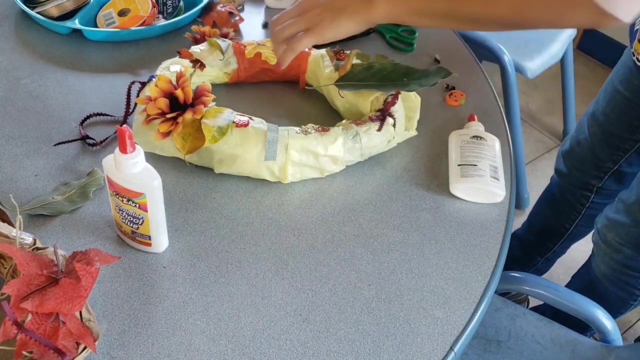 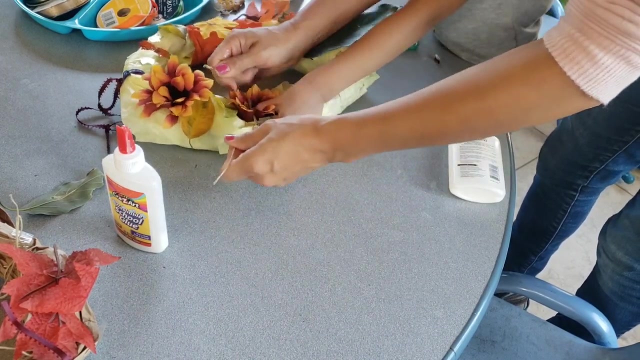 Okay, I'll help you. Hold on, hold on, Okay. Okay, I'll help you. Yay, As you may see, making this 3D art was very easy And, yeah, kids have a lot of fun being creative. 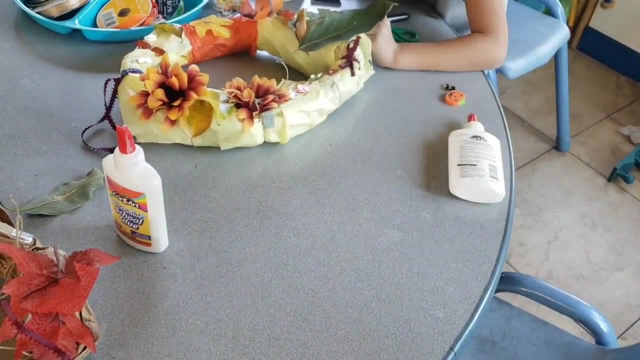 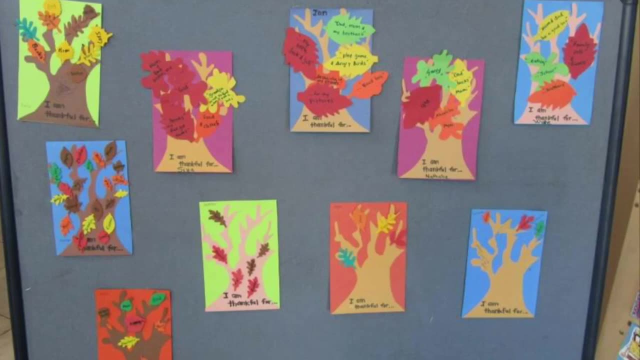 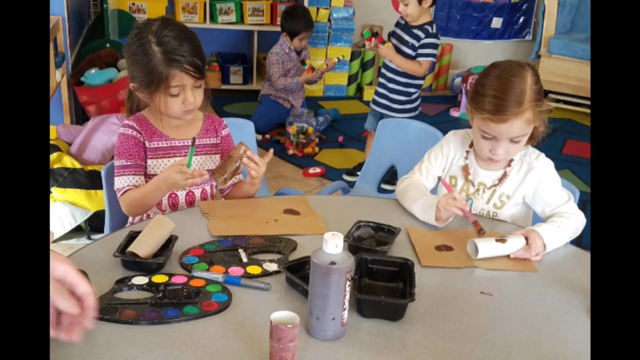 And it was a nice. this is that they could put in a home. Here are all their ideas of things you could do with your students making our thankful dream. Also, you could make turkeys that are 3D using paper rolls and adding the words. 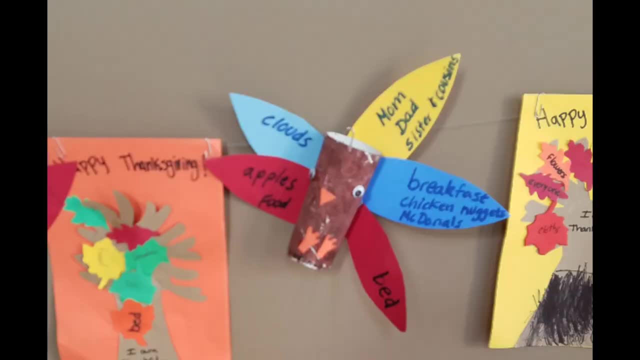 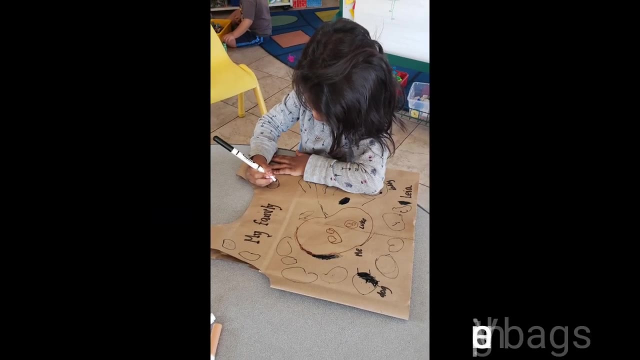 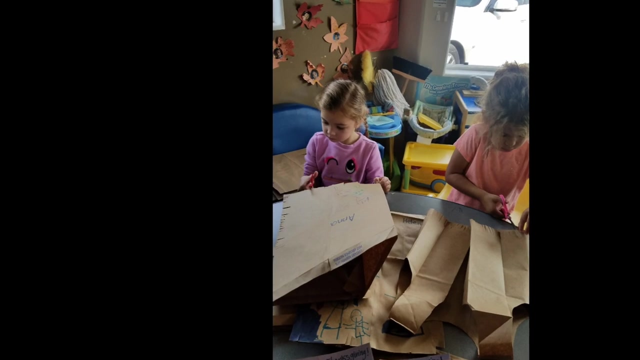 Why are they thankful? Mad activities for making numbers to put the feathers. We draw here a sentence giving. we talk a lot about family. Our students use these vests. We let them cut and draw pictures of their family in the back So they practice their fine motor skills. 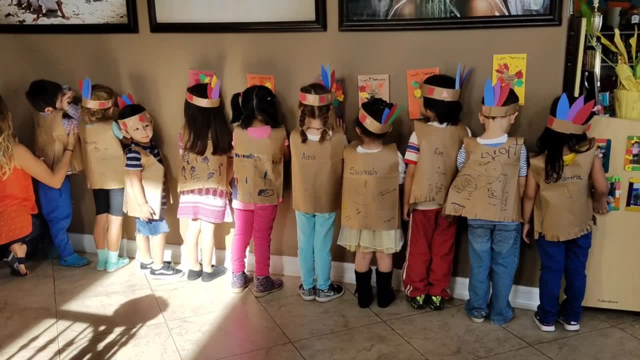 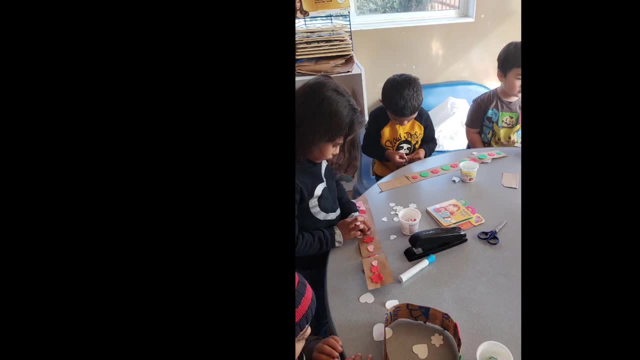 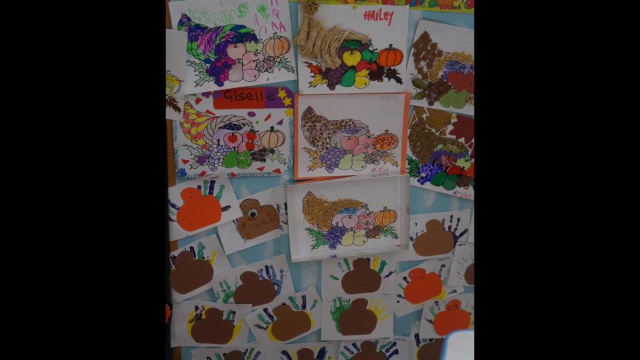 and also the creativity drawing their families as we practice how to make a face And we also make patterns. You can use their hats for them to make a pattern for their Indian hat. We also have done family projects or things that you guys could do at home.